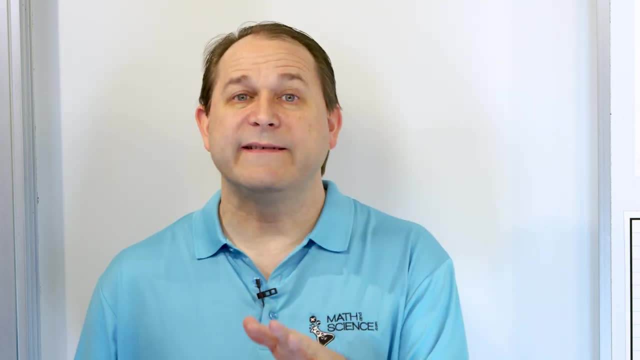 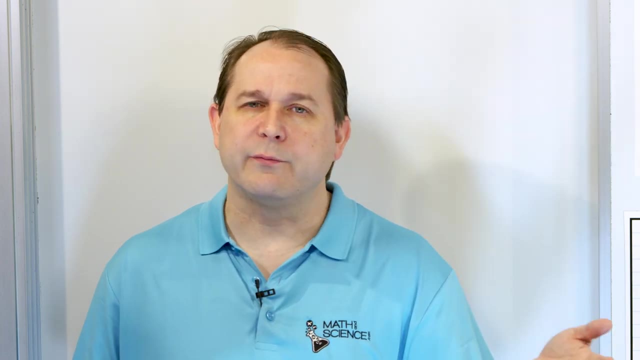 the intersection point. Now in this lesson- and that's going to be the solution in this lesson- we're going to solve these systems by just graphing them and then seeing if they intersect and where they cross. But in future lessons we're going to learn how to solve. 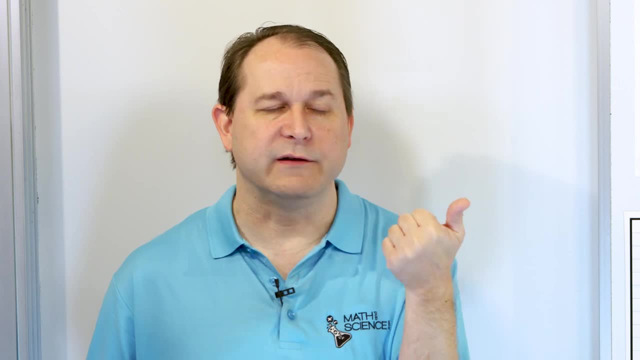 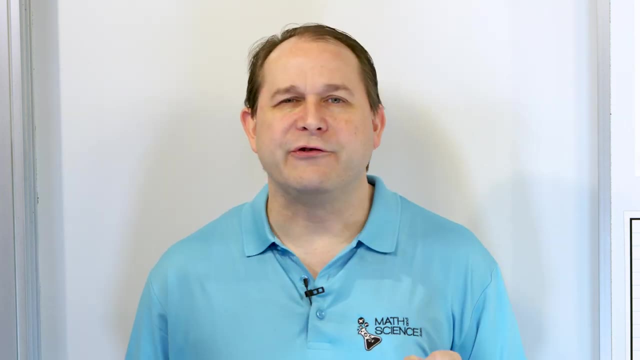 these systems without graphing, And we have a system called a solution method called substitution, And then we have a solution method called elimination. So just like different flavors, you know different flavors of you know whatever popcorn Some people like. 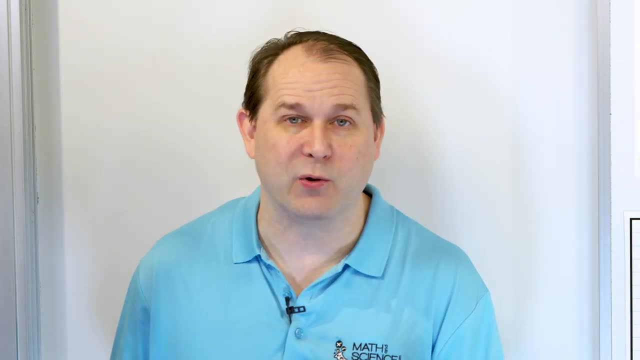 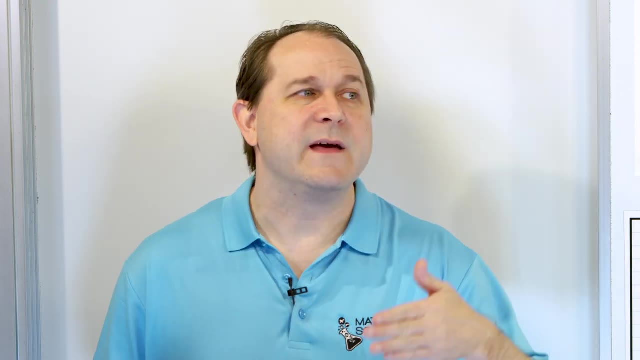 cheesy popcorn, Some people like salty popcorn, Some people like sweet popcorn. Okay, But it's all popcorn. Here we're learning systems of equations. Here we're going to learn how to solve it by graphing. Then we'll learn how to solve it by substitution. Then we'll 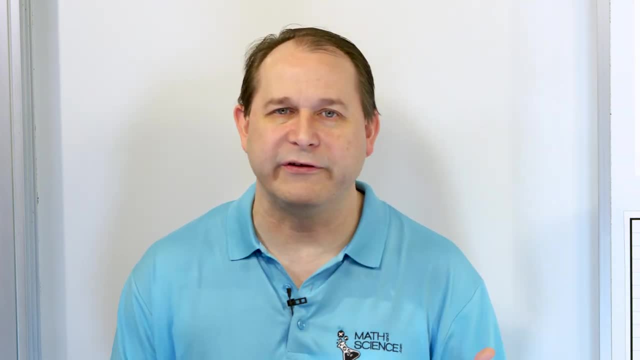 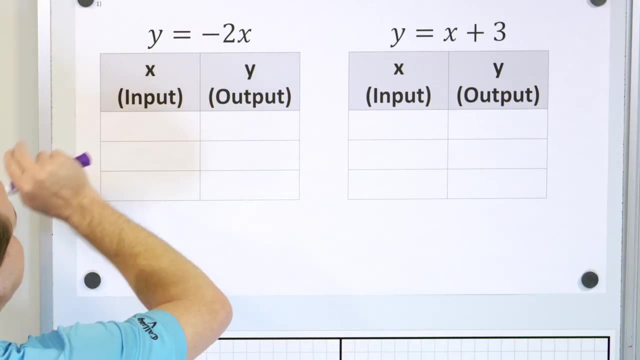 learn how to solve it by elimination, But we're still eating popcorn. We're still solving the system of equations, just different ways of doing it. So for our first set of, our first system is the are the two lines: y is equal to negative 2x and. 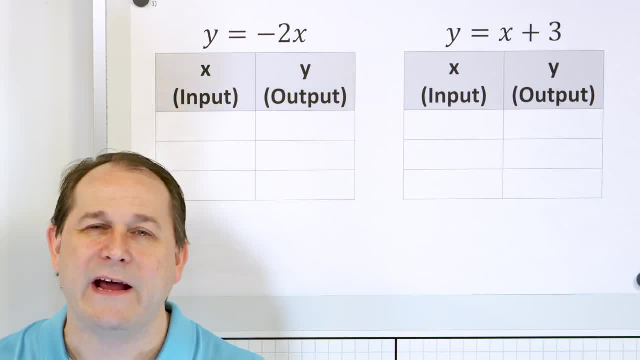 y is equal to x plus 3.. Now you can graph these lines any way you want to. For the first problem, I'm going to graph it using an input output table. We'll connect the dots and draw the line. And for the follow on problems, we won't use the input output table. We'll 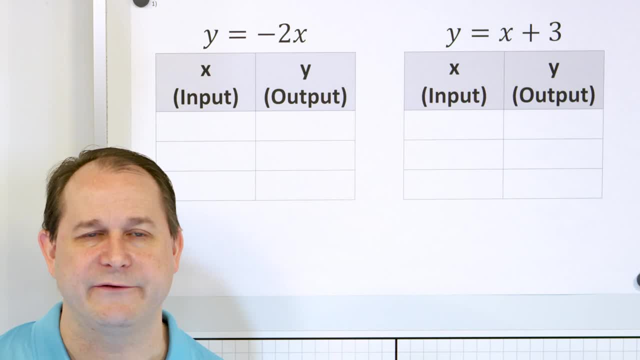 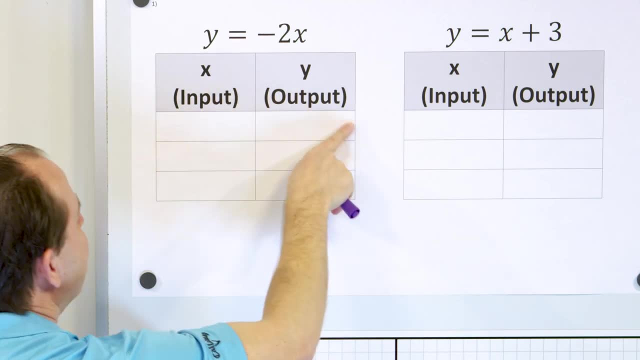 just graph it using the y intercept and the slope, which is a lot faster. So let's start off with our first problem. Here's our first line. We want to choose some input numbers for x and calculate the outputs. You can choose any numbers you want for x, literally anything You can even put. 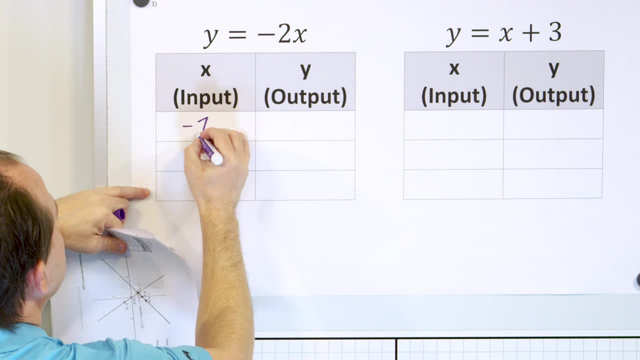 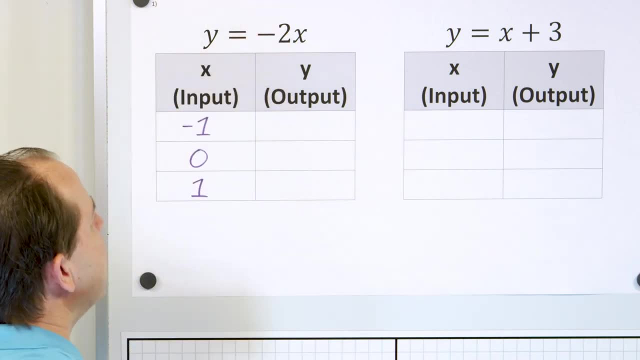 fractions here, if you want, or decimals Here I'm going to choose the number zero, negative, one for x, and then zero for x, and then one for x, And we're going to take each one of these three and we're going to put them in here. Now I'm choosing three points. We're 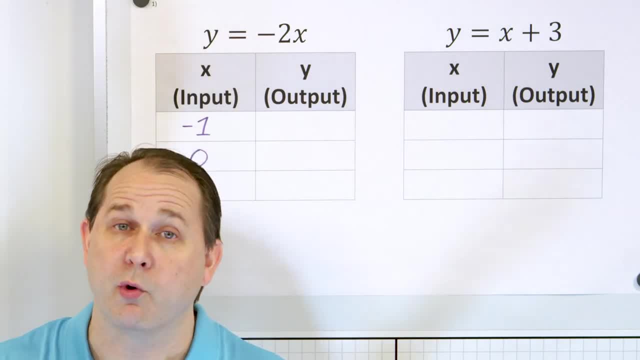 going to find three points for each line. I think that's a good number. You can choose more points if you want, But three points is nice because if if the line goes through it and it forms a line, then you know you've probably done the math correctly. So if I 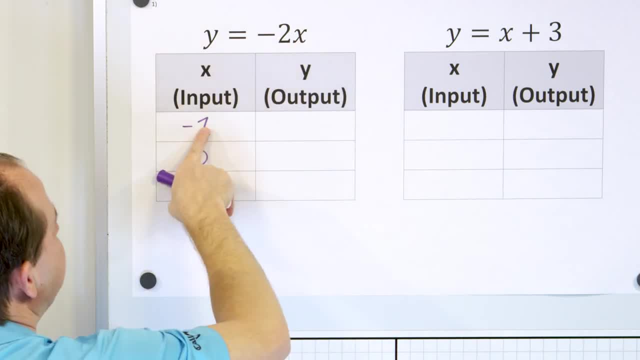 put negative one in here, it's negative two times x, which would be negative one. Negative two times negative. one is going to be a positive two, So the output would be a positive two. But if I put an x value of zero in here, then of course times negative two is again doesn't. 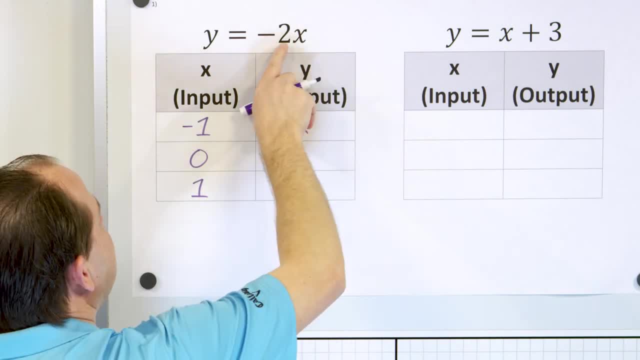 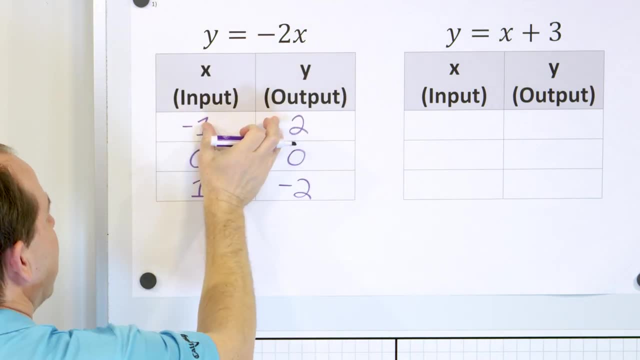 give me zero. What if I put a positive one in here? Negative two times positive one is negative two. So here's the input output table for the first line. Plot these points- x comma y, x comma y and draw a line. But before we do that, let's 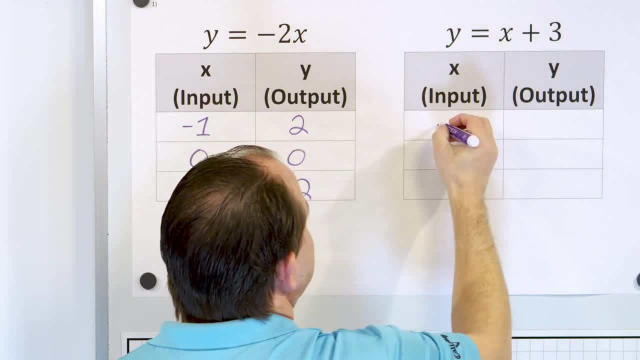 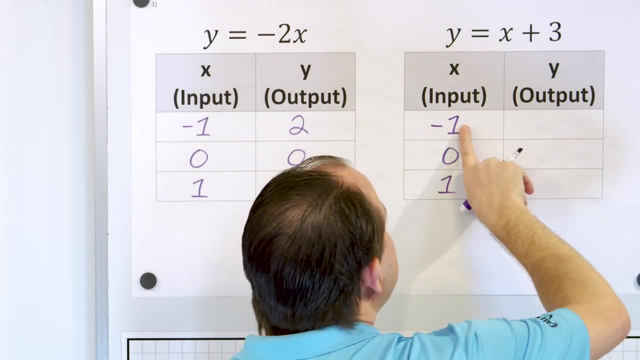 go on to the second equation of a line. Again, I can choose what I want to. I can put negative five here if I want to. I'm going to choose negative one, zero and positive one. They're just nice, easy numbers. If I put negative one in for x, then negative one plus a positive. 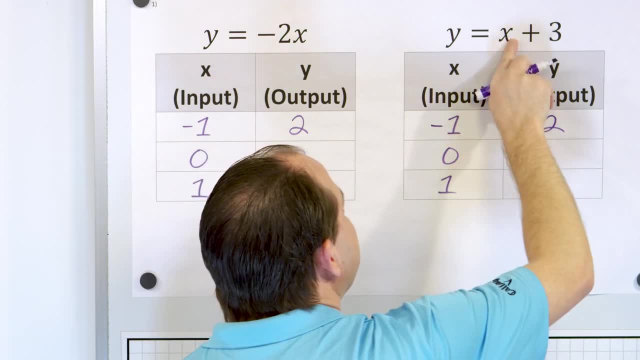 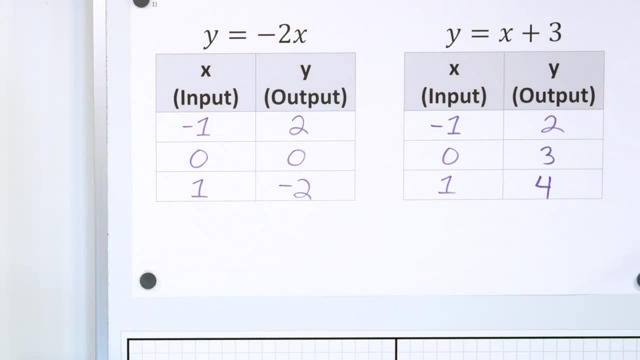 three is going to give me a positive two. If I put a zero in plus three is going to give me a three, And if I put a one in, one plus three is four. So you can always graph with input output tables. That's kind of the bottom line here. Let's take a look at the 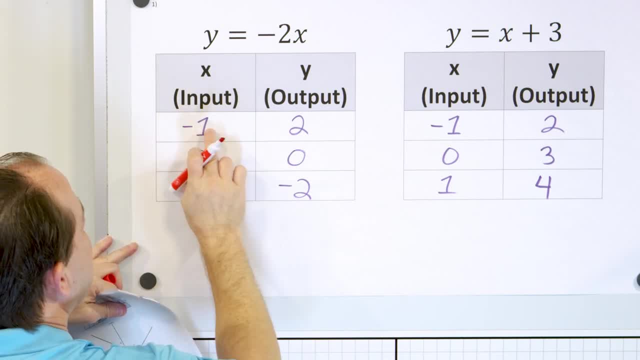 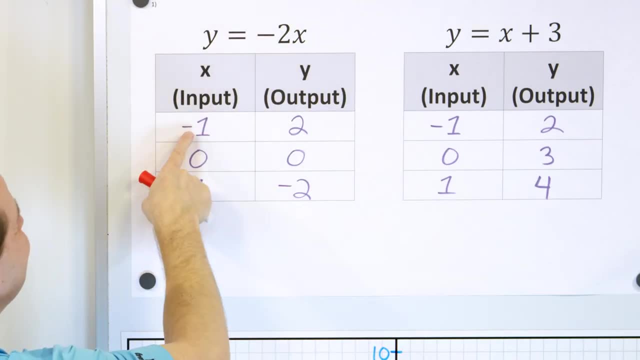 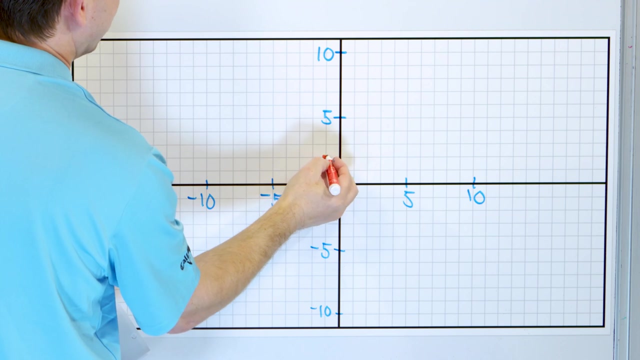 first one. The first line that we have is negative one comma a y value of two. So our first point from our first line is negative one comma positive two. That means we go over to the left: negative one and up two for a point that is basically right here at that. 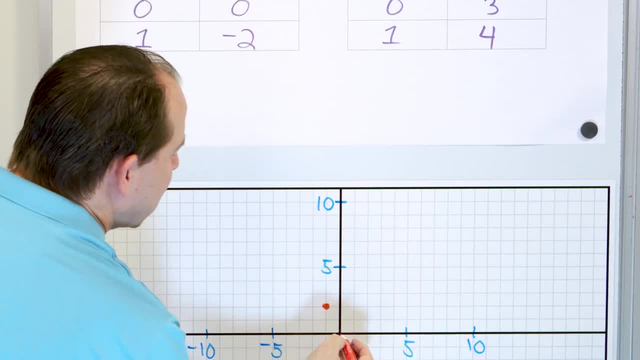 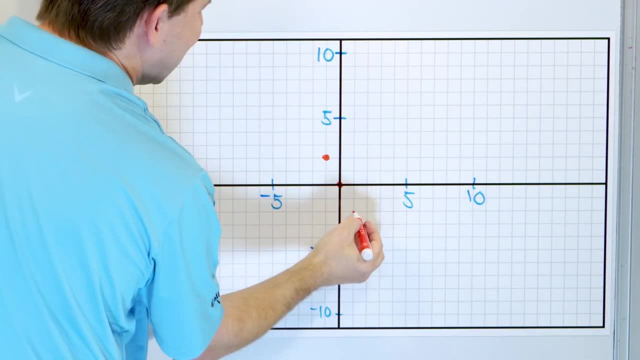 intersection point. The next point is zero, comma zero. That's right at the origin, right where everything intersects down here. And then one positive, one comma negative, two positive, one for x, negative, two for y is right here, And you can see that these three lines do indeed form, or these three: 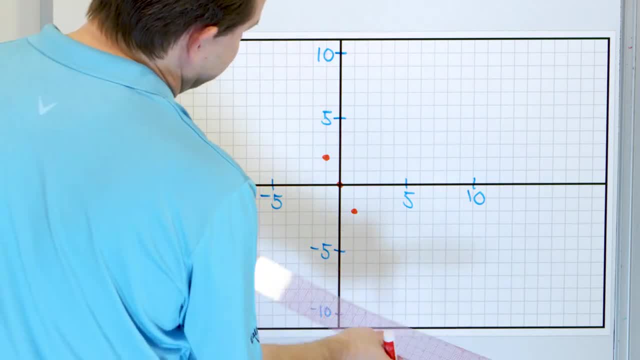 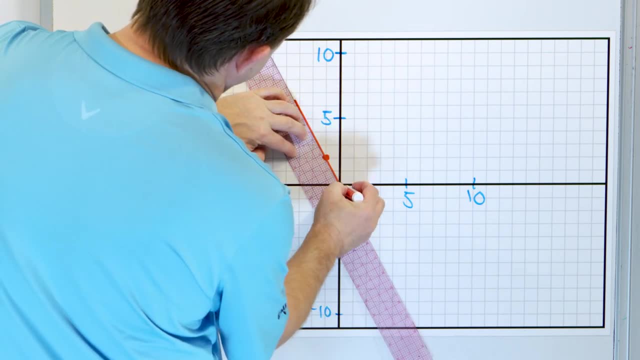 dots, I should say: do indeed form a line. Actually, I think what I'm going to do. yeah, let's just draw it right now. Let's just draw it right now. I was going to wait and draw both lines at the same time, but let's just draw it right now. So here is line number. 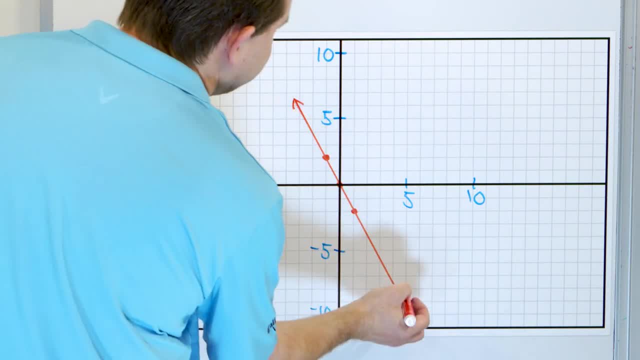 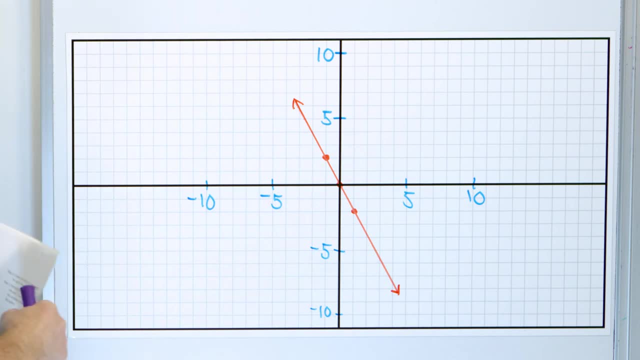 one, And I do recommend using a straight edge of some kind to draw your lines, because, basically, what we're going to do is try to figure out where these lines cross. If these lines are crooked or don't look great, then it's going to be tough. So here, 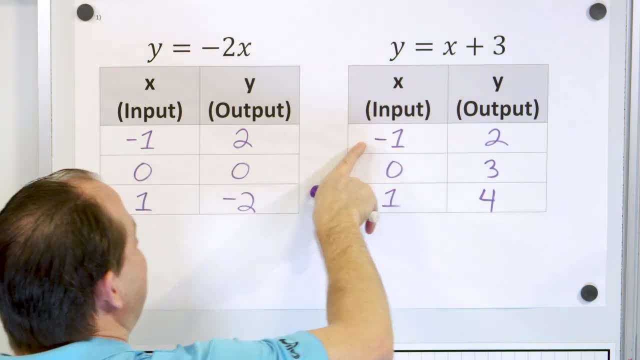 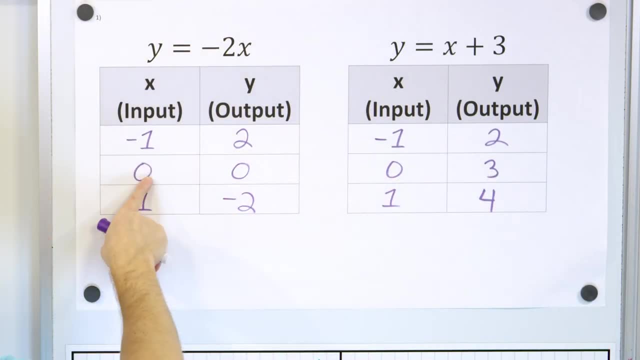 we have for line number two. the first point is the same as this point. It's just a coincidence: Negative one comma two. Negative one comma two is exactly the same point. Zero comma three. here, Zero comma three means zero, And then we go one, two, three. So there's point. 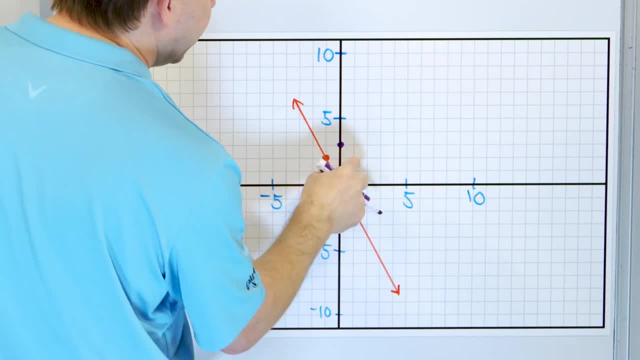 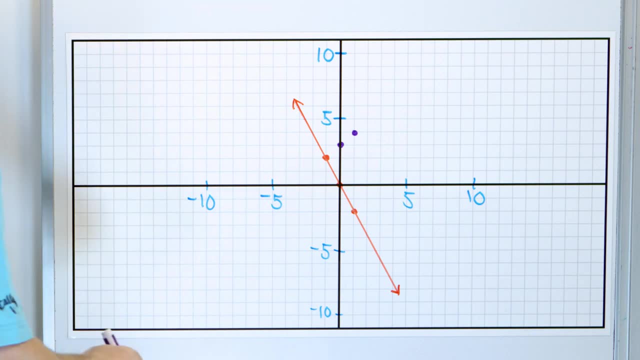 number two here, And then one comma four is one comma one, two, three, four right here. So the first point is this, The second point is this. The third point is this: I think you can kind of see where we're going with this and kind of like what the punchline? 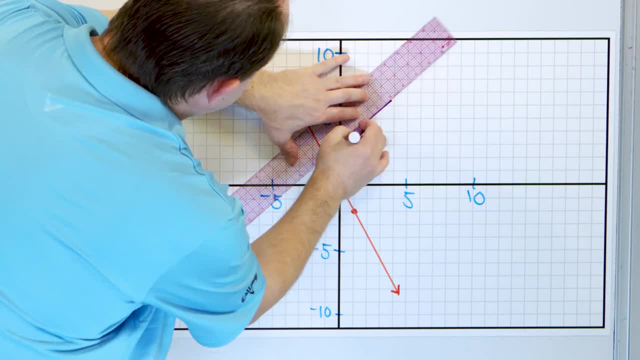 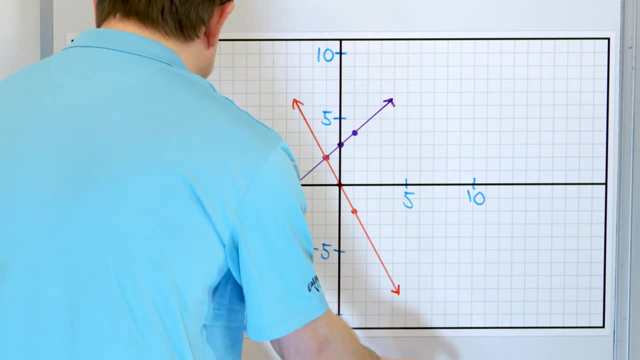 of this is going to be, but I'll go ahead and draw the lines anyway, And what you see is an intersection point right here. You can just see that the lines cross right at that point. All right, What is that point? If you look at this, that point is negative one comma. 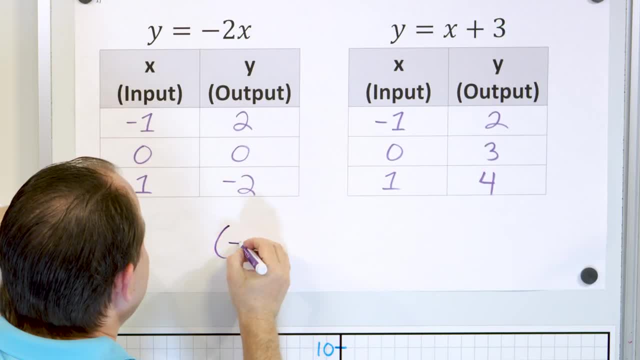 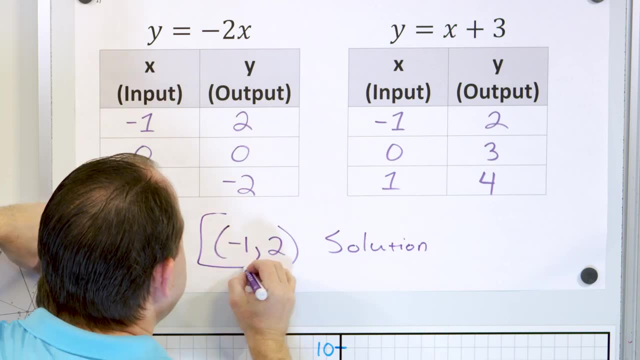 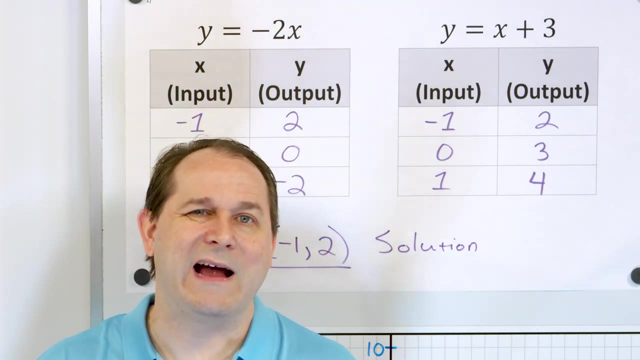 and then positive one, positive two, So the intersection point is negative one comma two is the solution. Now I want you to think about this from the big picture point of view when we learn how to solve regular equations. If I give you an equation like, Y is equal to two plus or. 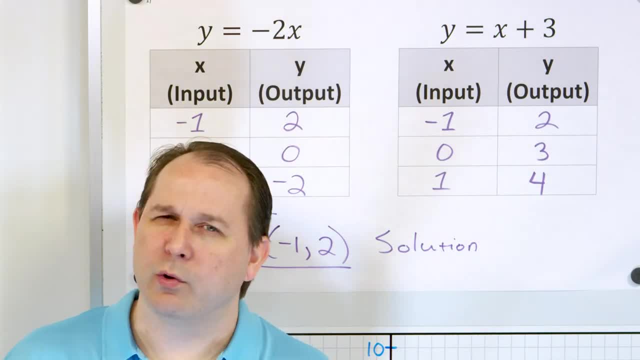 let's say two plus three is equal to X. right, Regular, old equation. you're solve for X, You're just getting a value for X. But when you have a system of equations, you don't just get a single value for X, You get an x and a y number and they form a coordinate. 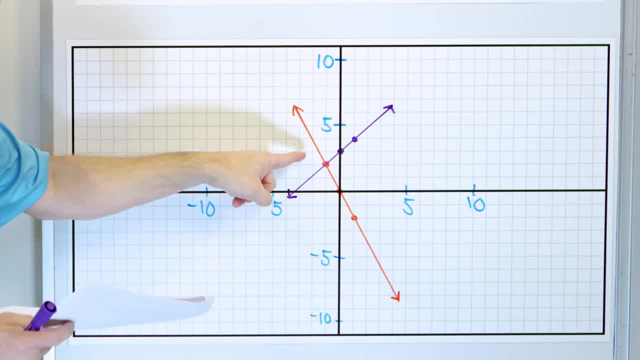 pair, But it's still a single point. Now these lines crossed at one point, And so there's going to be one solution. Most lines are going to get: awhen is an incoming line, And then it's just going to be a single equation, All right. So now that that's bigger, those lines are. 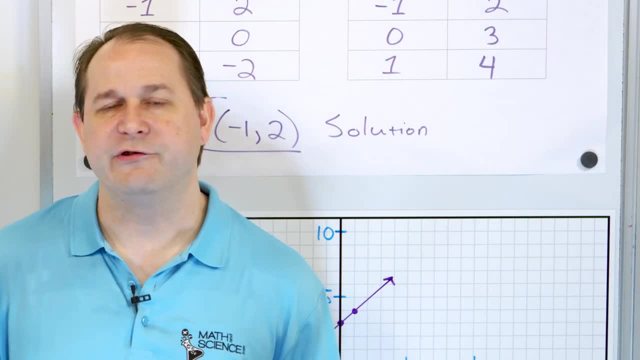 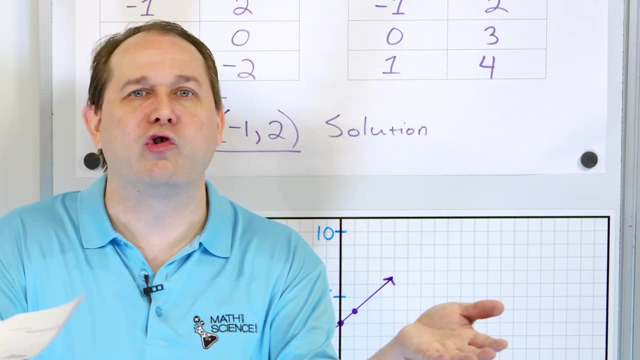 lines, they're going to randomly cross somewhere and that's going to be the solution. The only time you're really not going to have a solution at all is if the lines are totally parallel and they never cross. Even if they go on forever, to infinity, they never cross if they're parallel. 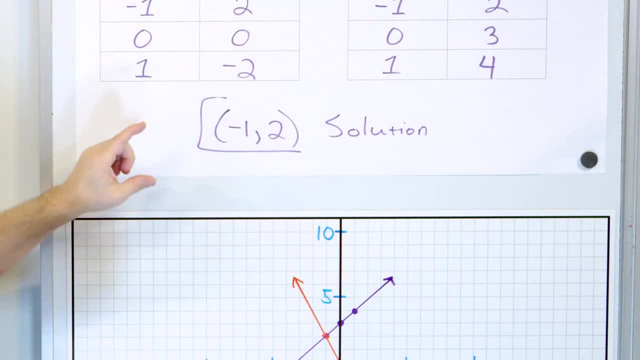 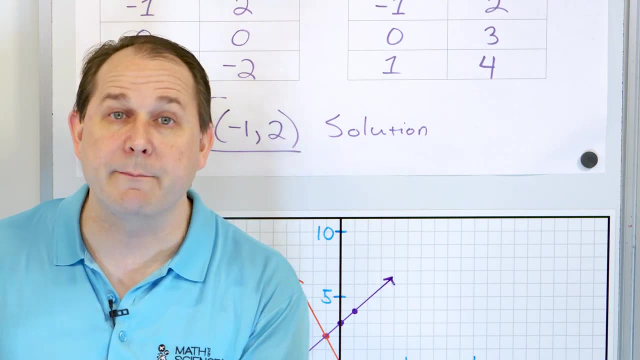 And in that case we say there is no solution. But here what you do is you circle. the solution is the point x comma y. So whereas when we solve a regular equation we're just looking for a number, when we solve a system of equations we're looking for an x- y point. So the solution 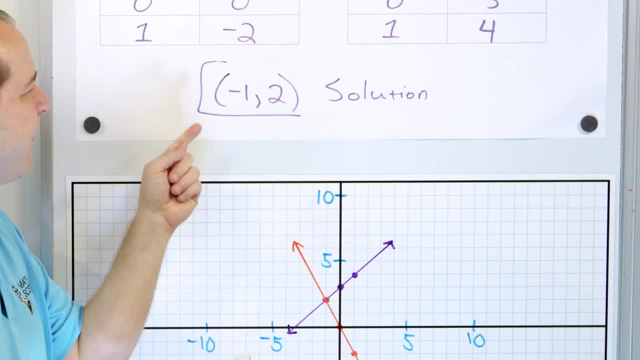 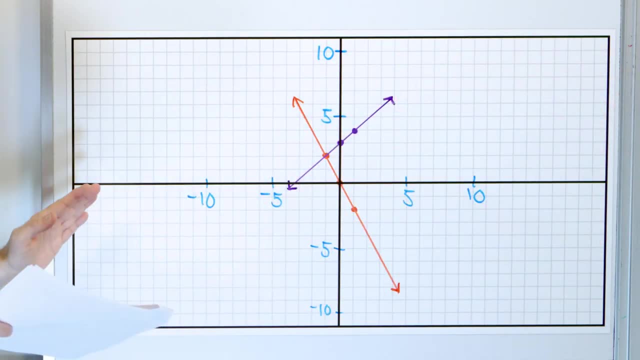 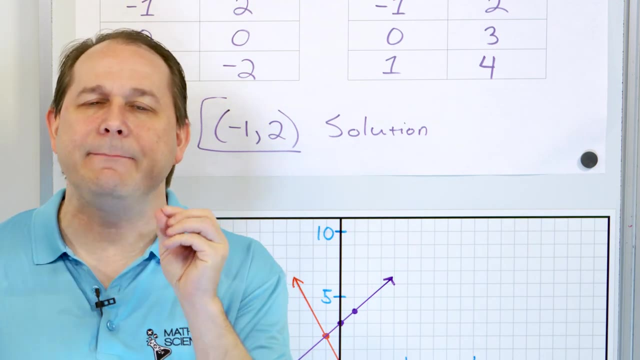 itself is actually the point 1 comma 2.. And again, the reason this is a solution is because the point negative- 1 comma 2, is the only point in this entire grid that, at the same time, satisfies both lines at the same time. And when I say satisfies it, I mean that this: 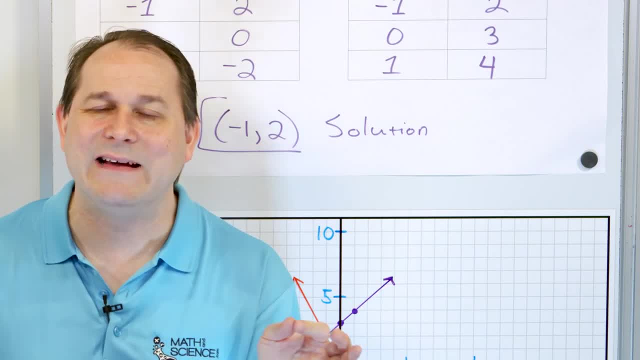 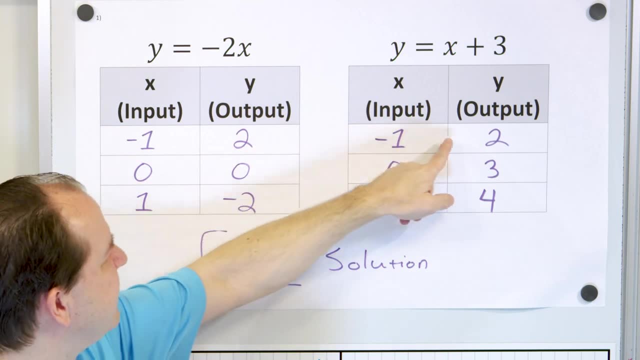 point is true for both lines, because this point lies on both lines. You can see this point is in the table. It's in the tables actually here. But even if we chose different, like if we didn't choose negative 1 here, we wouldn't see this point in the table, but we would still see the intersection. 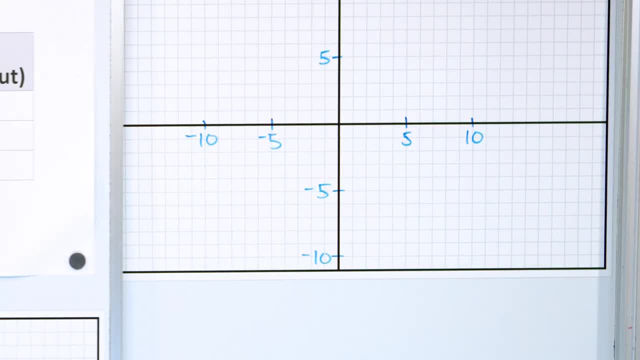 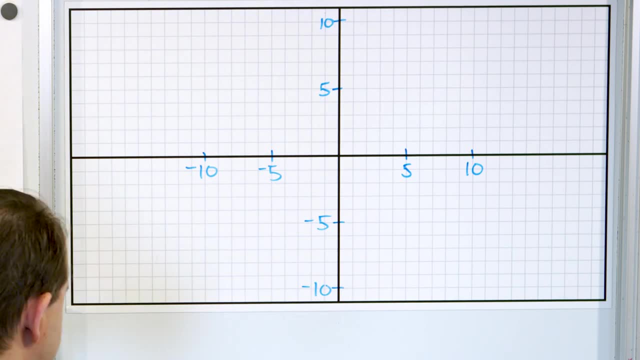 point being in the same place there. All right, Now for the follow-on problems. we're not going to do an input-output table anymore, because, even though it's very nice to do that and learn about it, it is not the fastest way to graph equations. 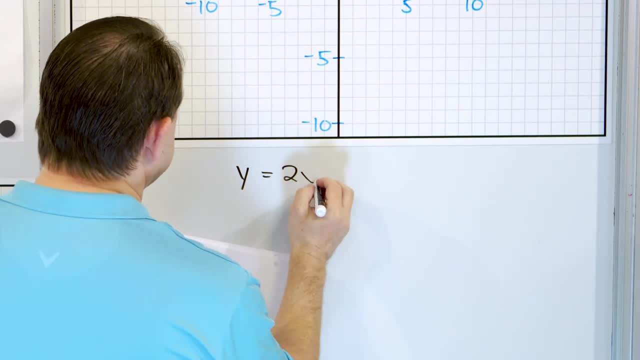 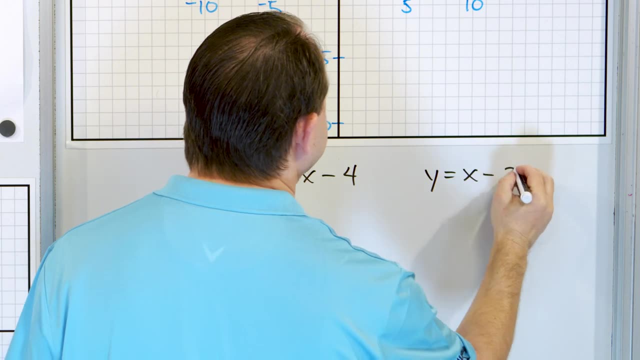 So let's take a look at problem number two. How about? y is equal to 2x minus 4.. And the next equation? I guess I'll write it over here: y is equal to x minus 2.. You can graph them. 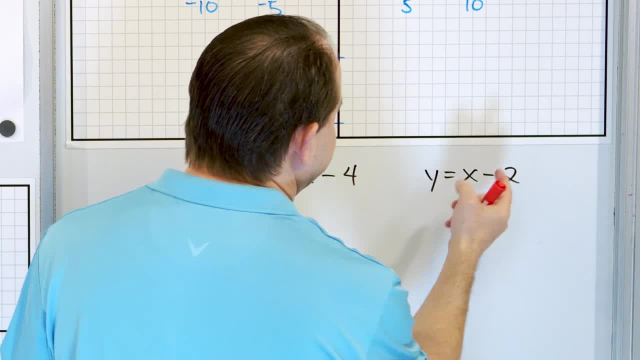 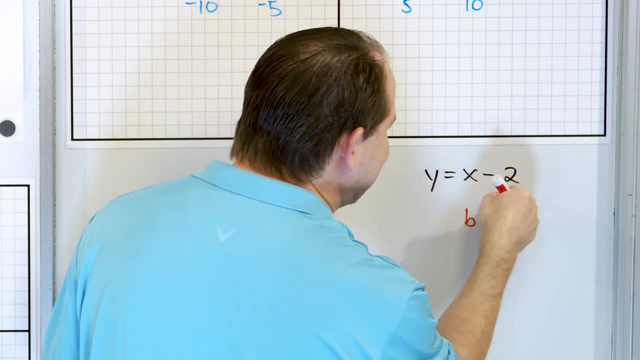 in any order you wish, And so let's just graph this one first. What is the y-intercept of this guy? The y-intercept of this guy is negative 2. because it's x, You can think of it as plus a negative 2.. So there's the y-intercept. 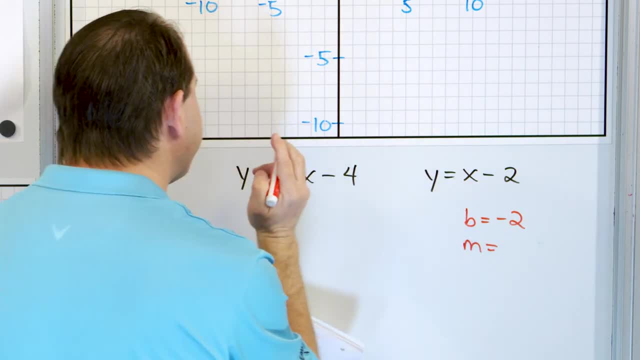 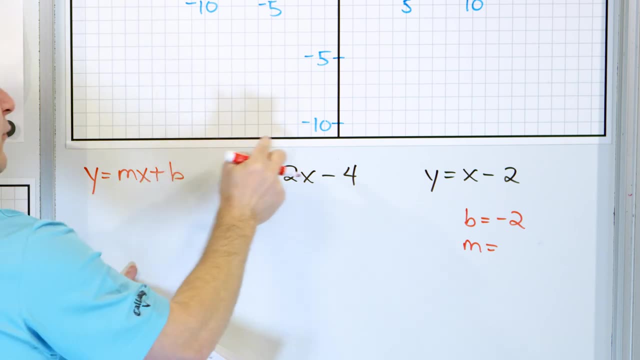 What is the slope? The slope is whatever is in front of x, because, remember, all lines have the form mx plus b. The y-intercept is negative. 2. The slope is whatever is in front of x, But there's an invisible 1 there, so the slope is 1.. When you get a slope of 1, that means 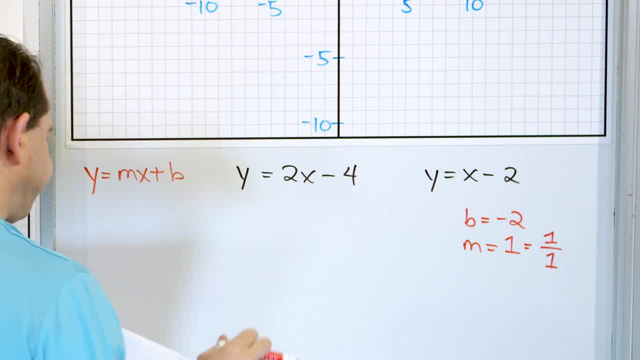 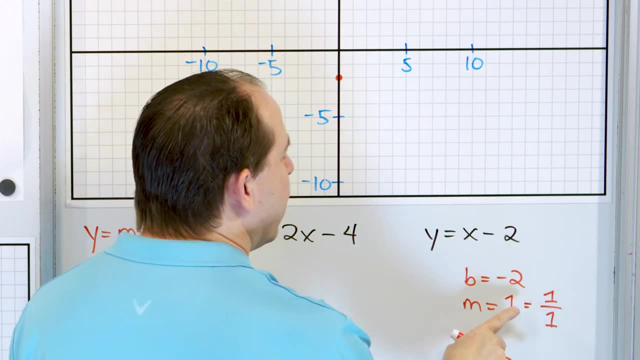 a rise of 1 and also a run of 1.. So all we have to do is figure out where the y-intercept is. here It's at negative 2, so I put a dot there And then we go. slope of 1 is up, 1 over 1.. And if you do it, one more. 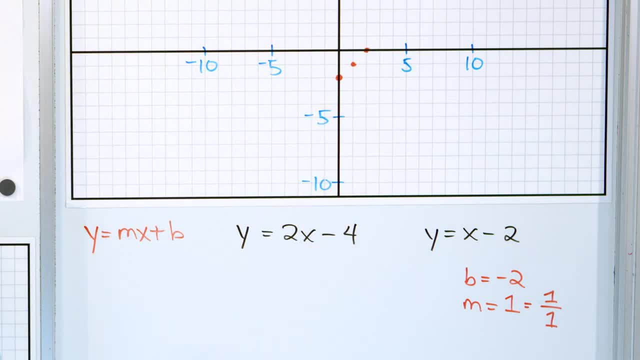 time up 1 over 1.. And there we have three nice points and it's going to be easy to draw a line through those three points. So I don't know where this line is going to be consected. 3 has a power equipped next. So if I particularly don't know where the y-intercept of this guy is, 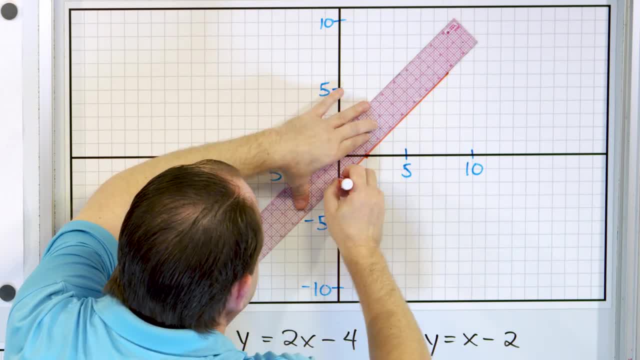 I'm probably going to have y cough quarantined. These goes into the bottom right corner and there's a going to cross the other one, or if it even is going to cross at all. So I'm just going to draw a nice long line through the whole thing And hopefully I'll catch the intersection point. 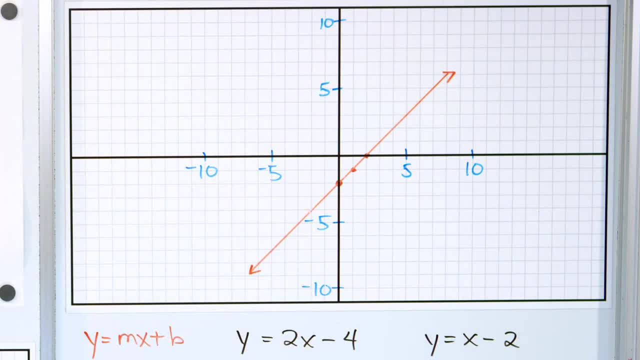 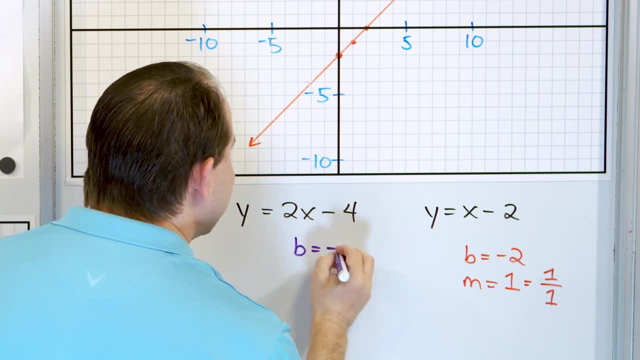 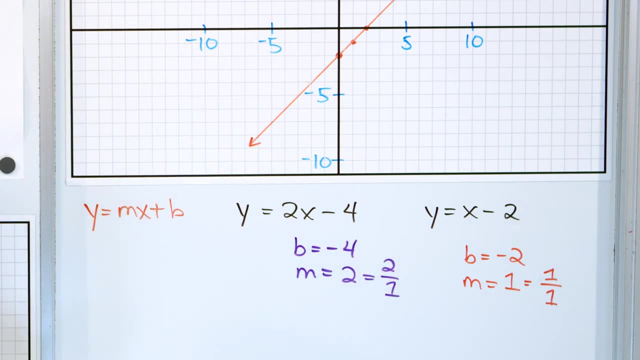 for the other line, All right. So what is for the other line? what is the for this line here? what is the y-intercept? Well, the y-intercept is negative four, right here, And the slope is whatever's in front of x, which is two, which is a rise of two and a run of one. That's what a slope. 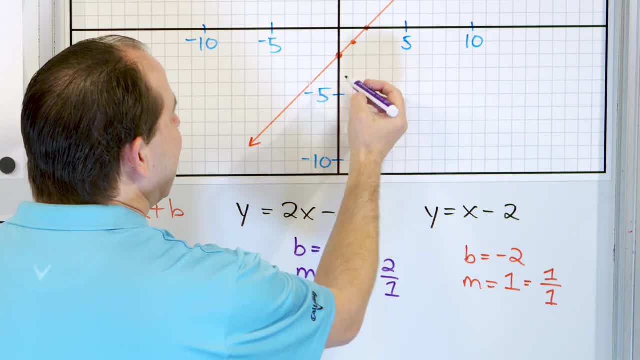 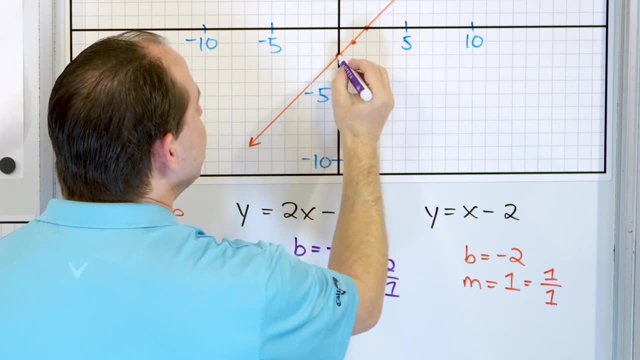 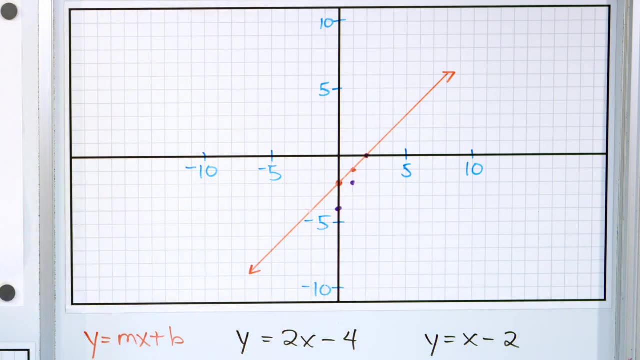 of two is. So we go to the y-intercept of negative four, which is right here, right above negative five. So negative one, negative two, negative three, negative four, And the slope is two. That up two, and then over one, which is right here, actually right on top of that, And so then I can. 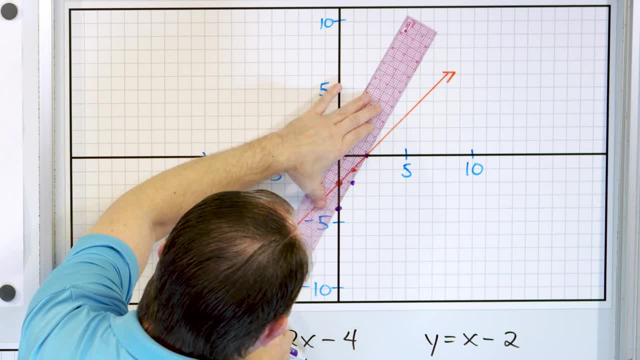 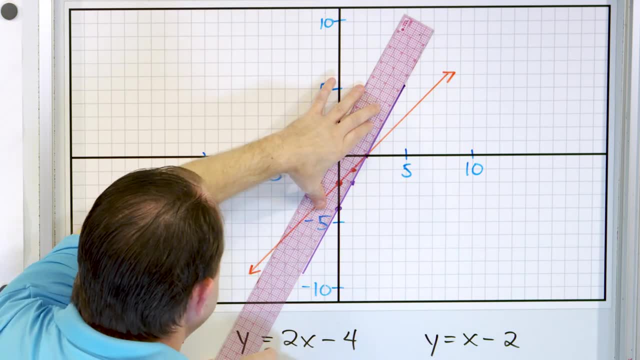 draw a line through these points. So there's a point, there's a point and there's a point, And I think you can all see where the intersection is going to actually be right, And so I'm going to draw a line through this point And I'm going to draw a line through this point And I'm going to 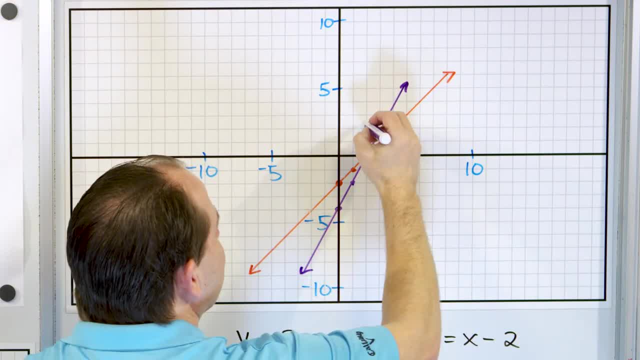 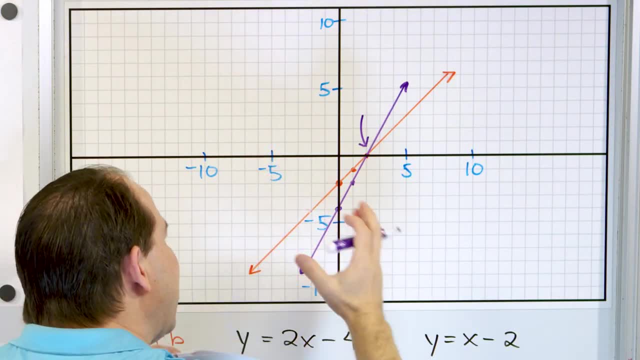 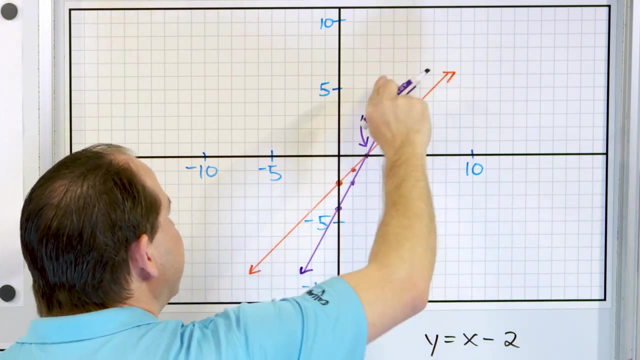 And so we have the two lines right here and the intersection point is right here. That's where the lines cross. That is the only point in this entire plane that is present in the red line and at the purple line at the same time, because this point is true and satisfies both of these. 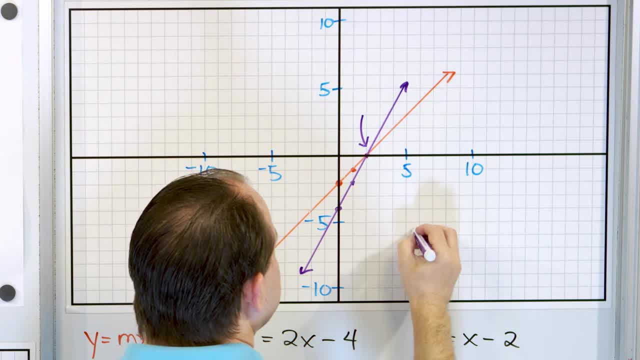 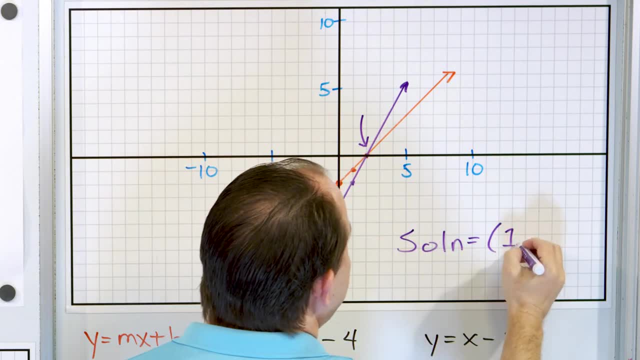 lines at the same time. So it is what we call the solution. So the solution of this, the solution is equal to the point. And what is this point? It is an X of one and a Y value of zero, because it actually lies on the axis. 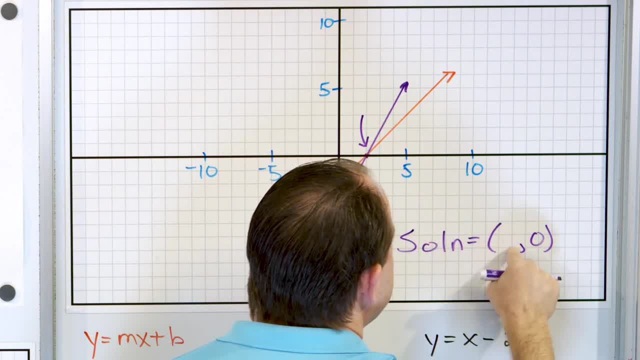 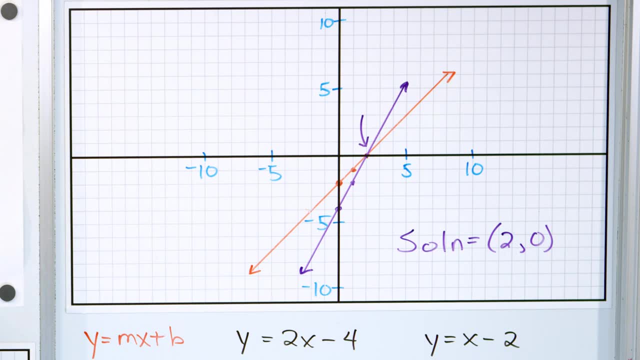 Actually not an X point of one, sorry, one two. It's an X point of two there. So two comma zero, two for X and zero for Y. So there is the solution, All right. So you can see how straight lines are going to help you a great deal here. 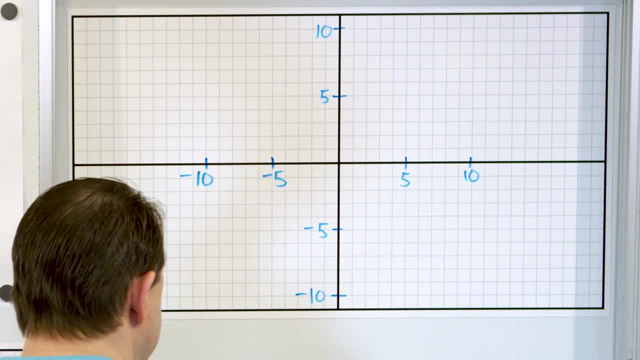 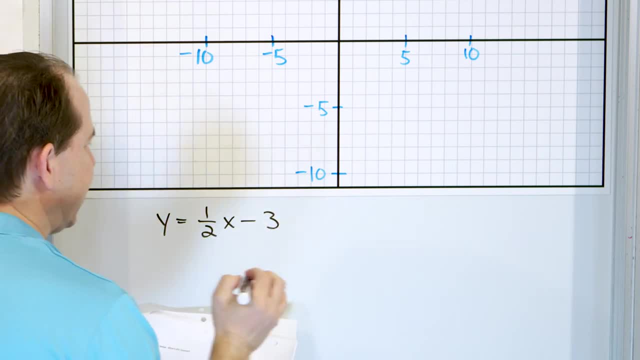 Let's take a look at our third one here, And the first line is going to be one half X minus three, And the second line is going to be negative X plus three. So you can graph whatever you want, whatever order here. The Y intercept is the negative three, which is over here. 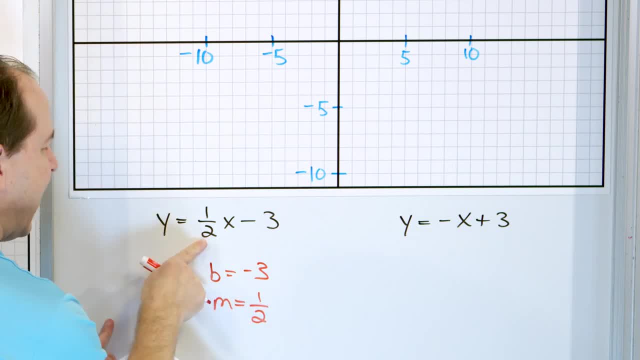 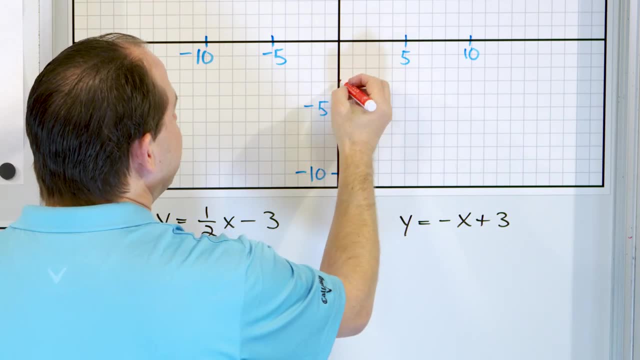 And the slope, which is one half, is whatever's in front of X: rise over run. So let's go and take a look at this. The Y intercept is negative three. That means I go negative one, negative two, negative three. put a big fat dot right there. 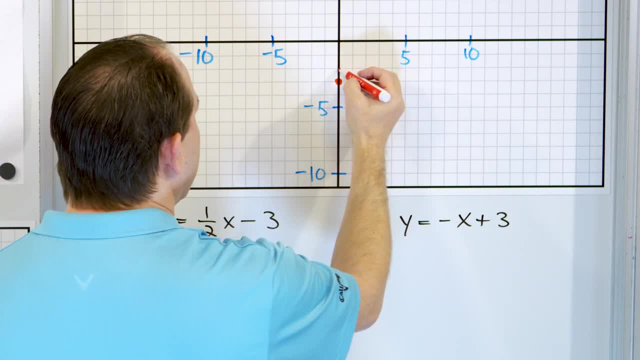 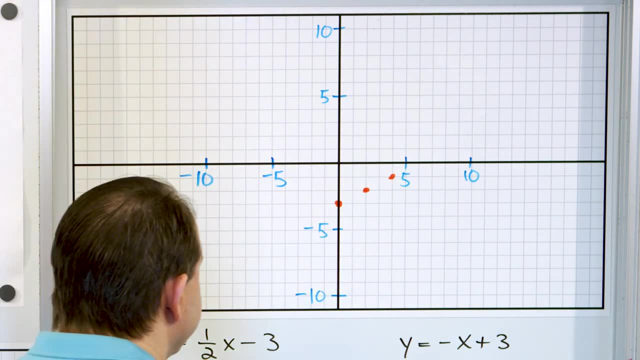 Rise of one run of two from here up one over two. That means my next dot. My next dot is here, up one over two. My next dot, again, is right here. So I grabbed my straight edge. I don't know where the crossing point is going to be, or even if it is going to cross the 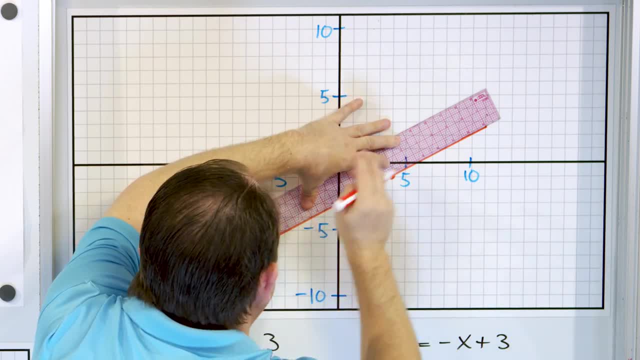 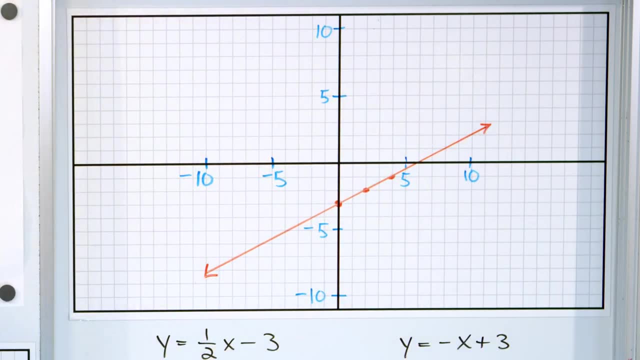 other line. So I'm just going to draw a nice straight line, nice long line, through all three of these points And there is my line for for the first equation that we have. All right, Let me just double check my work so far. 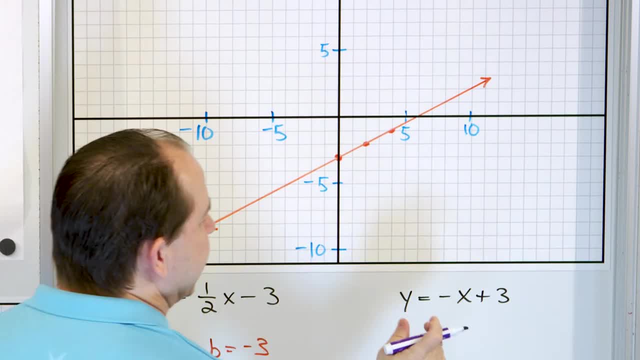 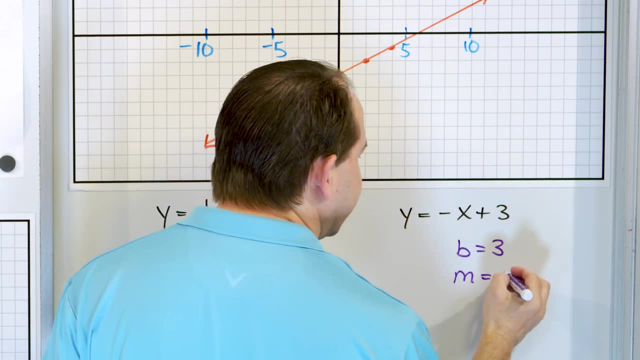 All right, Now what about the second line? What is the Y intercept? It's a positive three right here, And the slope is whatever's in front of X. There's a negative sign here, which means the slope is negative, one which is a rise. 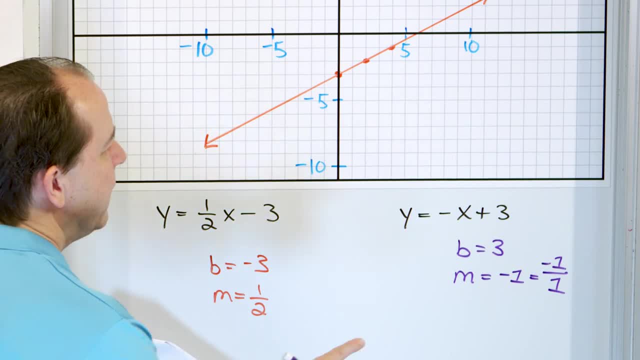 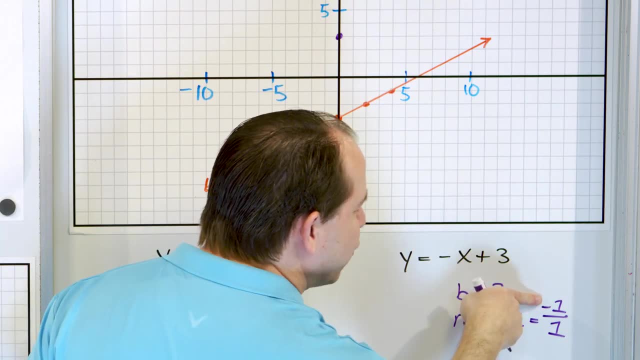 of negative one and a run of one. That's how we think about it. Y intercept is at three, one, two, three right here, And we go see, since it's a negative, we rise down one and go over one. 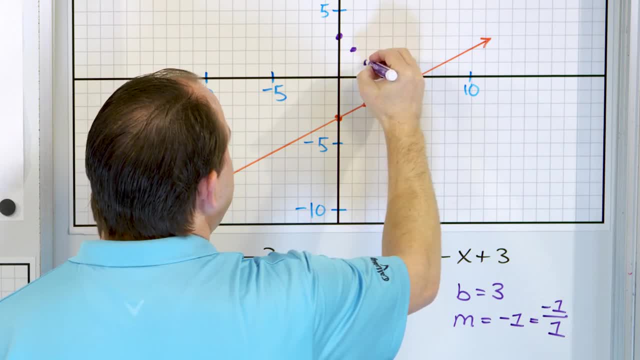 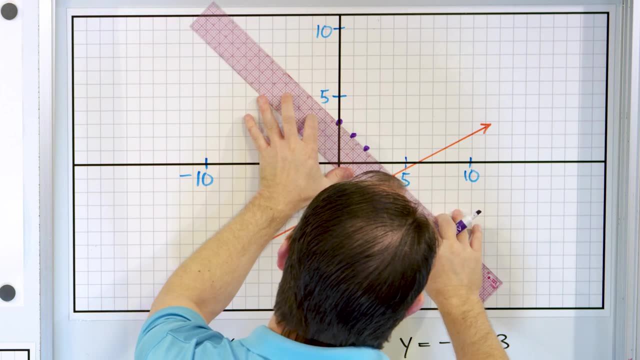 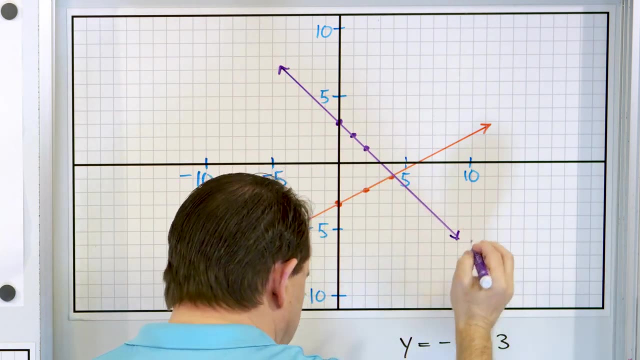 Down one over one, And then from here down one over one, And now I have enough points to draw a nice line. All right, So let me line this up through here and I'm going to draw a nice line through there. Now you can tell that my graphing is not perfect, because if you look carefully you can tell. 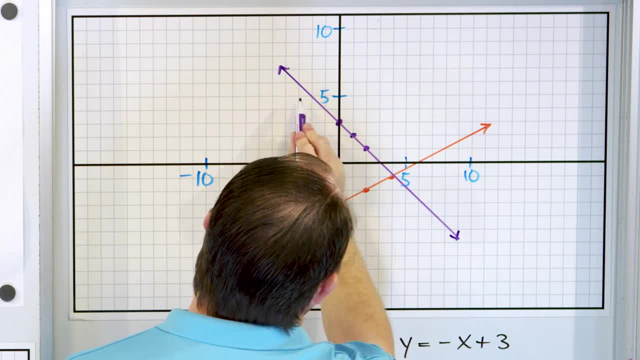 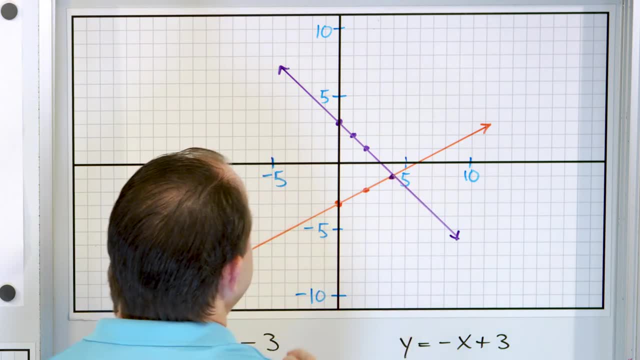 that the point is right here at this intersection, but because my line was not actually perfectly through exactly the crossing of all these. it looks like it's a little bit higher, But this point, right here is the point, right at that intersection point, is the solution. 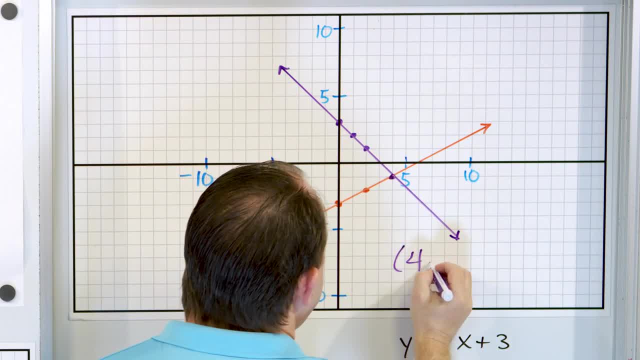 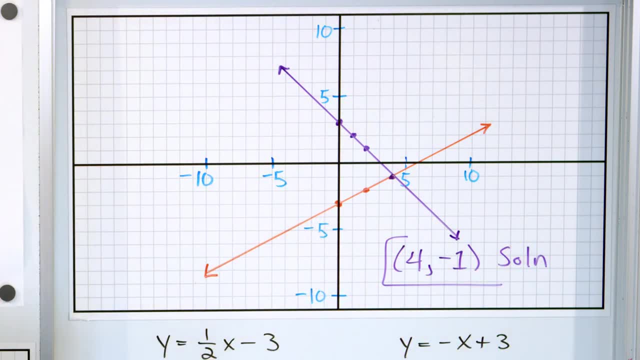 It's One, two, three, four And Y goes down. So that's negative one And this is the solution. So you circle this: four comma, negative one. That's the solution. Again, this is the point. It looks like it's not quite right. 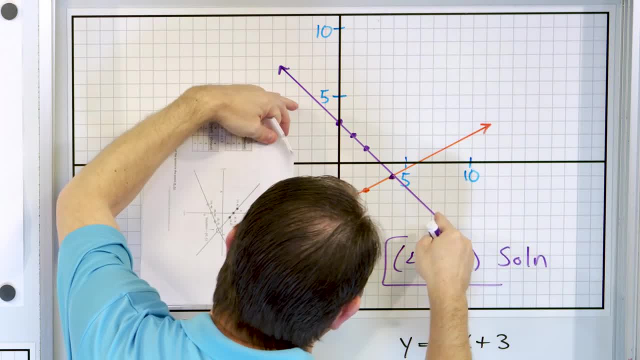 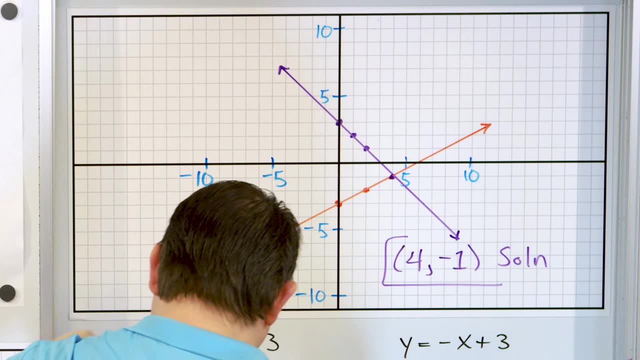 It looks like it's a little low. That's because my red line and my purple line are just not perfectly like. you can see that that purple line is a little bit higher than it should be. I should have tilted it down. It would have gone right through that guy. 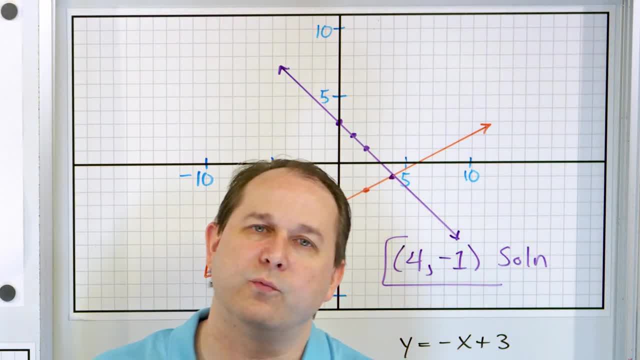 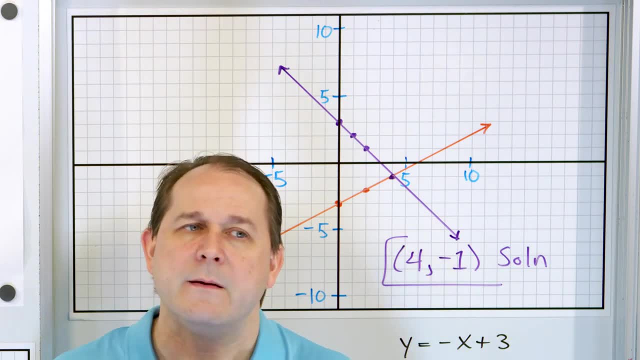 We do have one more problem, but I do want to share with you that this is reason why we learn. We learn these systems by graphing, But in real life we don't usually solve them by graphing, because the graph is only going. 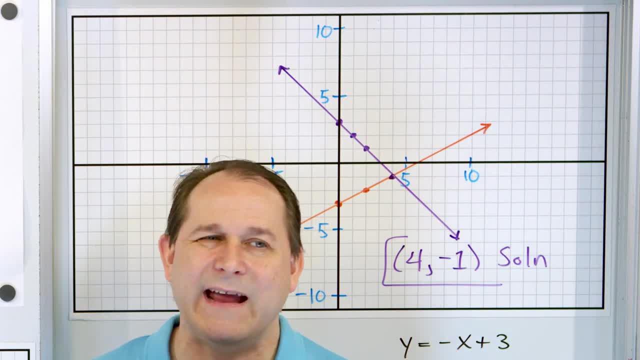 to give you a solution. as perfect as your lines are drawn- and we can never draw perfect lines None of us can Like- even with graph paper, you can't draw it perfectly right. So graphing is great. It's good graphical to help you understand what you're doing, but it's never going to. 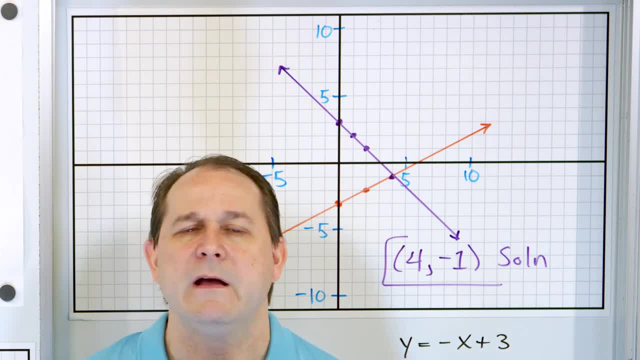 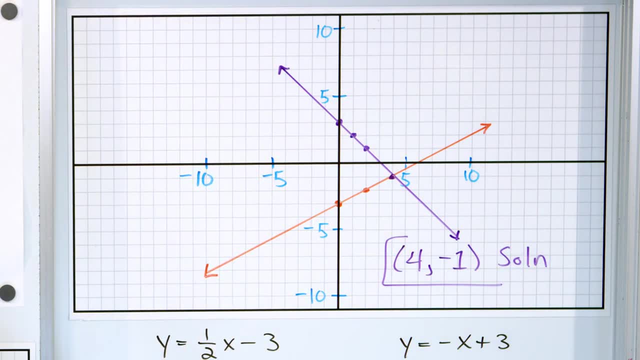 give you super accurate, super amazing precision. okay, So we learn it, but really in real life we learn the other techniques we're going to learn later to actually solve these guys. So the solution of this is four comma negative one. I'm going to erase this. 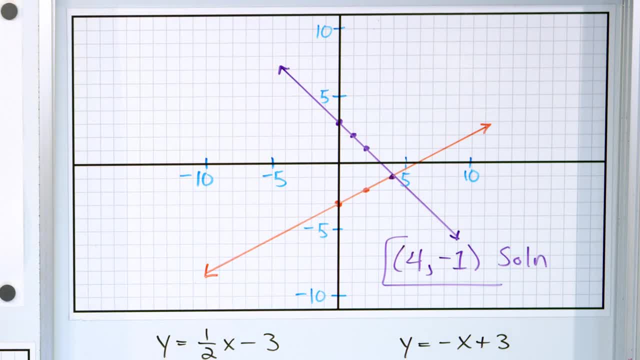 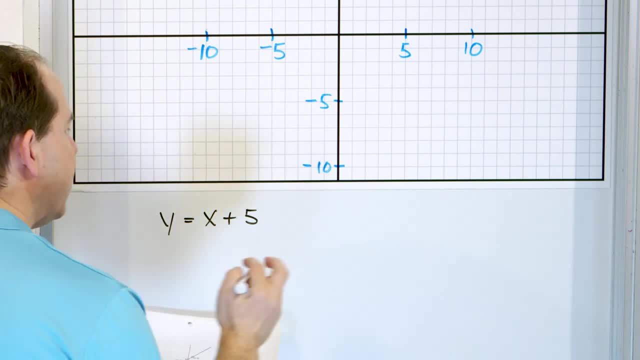 We do have one more problem and we will wrap it up and call this lesson completed. All right, here is our last problem. The first equation is X plus five. Y is equal to X plus five. Second equation is: Y is equal to X minus one. 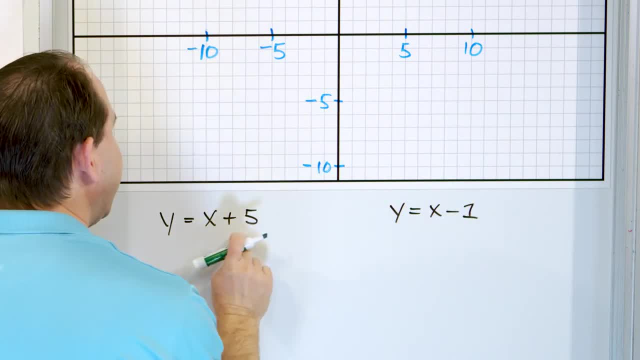 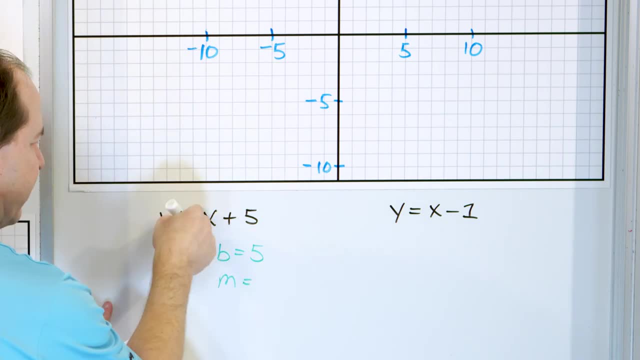 All right, so let's take a look. What is the Y intercept of this first guy? That's going to be five, because the five is sitting over here. The slope is whatever is sitting in front of the X, which is an invisible one. 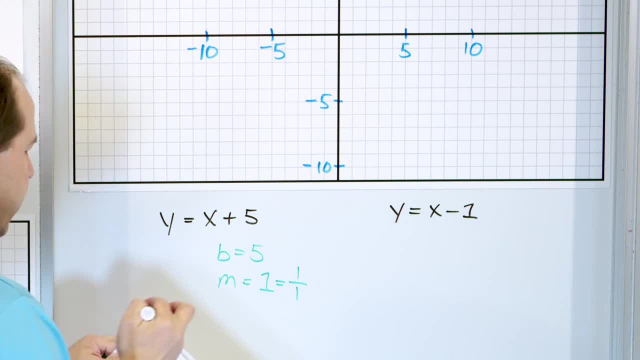 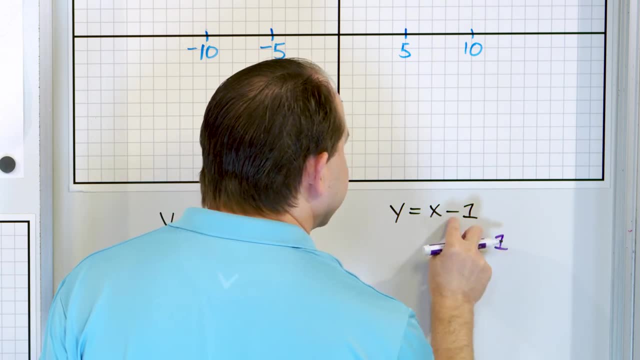 So the slope is one which is a rise over run. one over one. right now, over here we have what did we have? The Y intercept is negative one because it's sitting here and the slope again is one because that's what's in front of X. one over one. 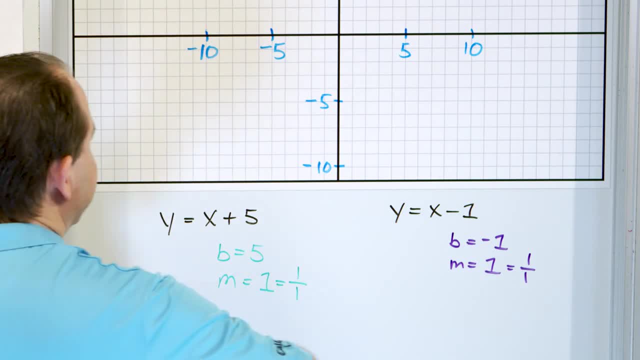 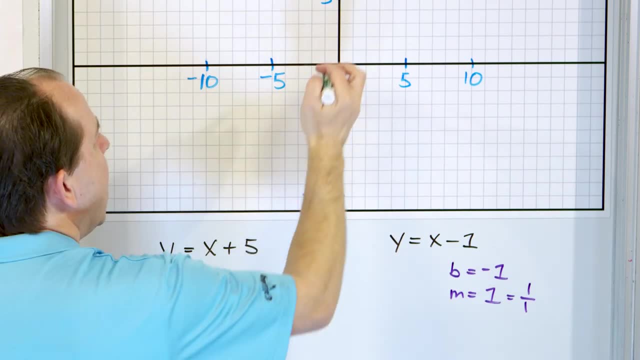 So let's graph these guys and see what we have. So, with a Y intercept of five, that means the Y intercept is right here, up at positive five, and the slope is one up one over one. Here's the next point: up one over one. 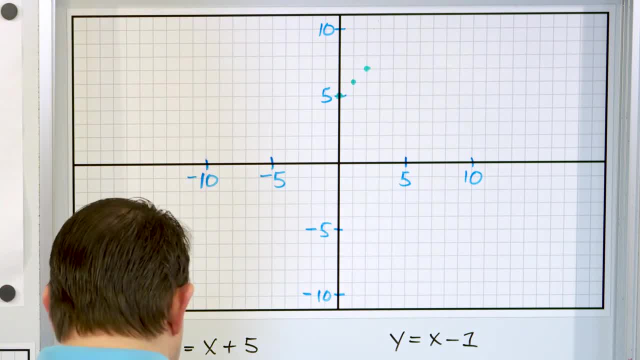 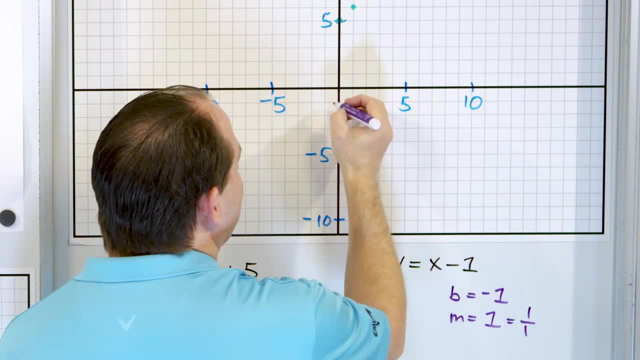 There is the next point. all right, and I think what I'm going to do is put my next points up before I draw my lines. What is the Y intercept here? The Y intercept here is negative one. That's way down here and the slope again is one. 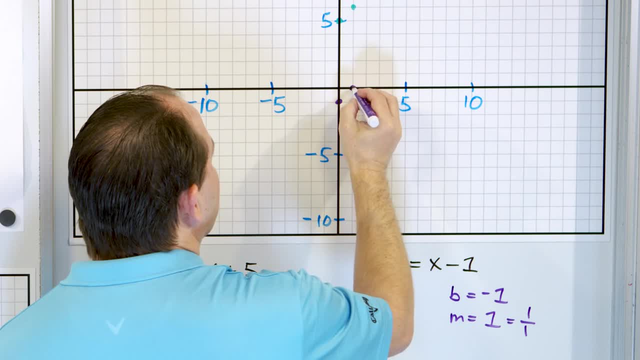 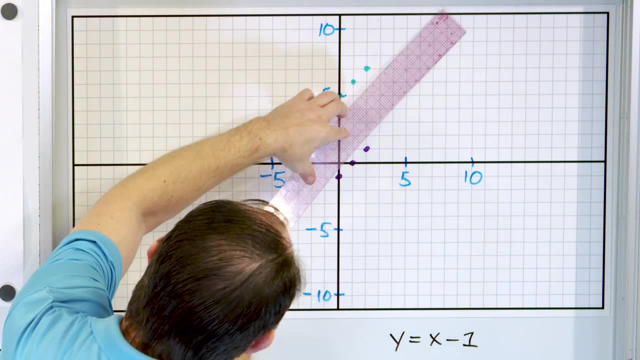 So it's rise over, run one over one here. rise one, run one like this. So let's draw these as good as we can. It's not going to be perfect, but that's okay. We're not after perfection, We're just after trying to get an idea. 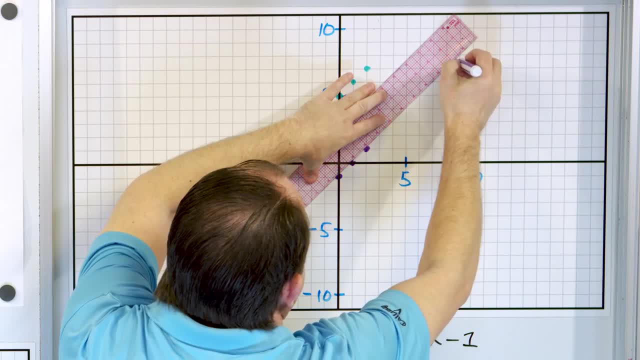 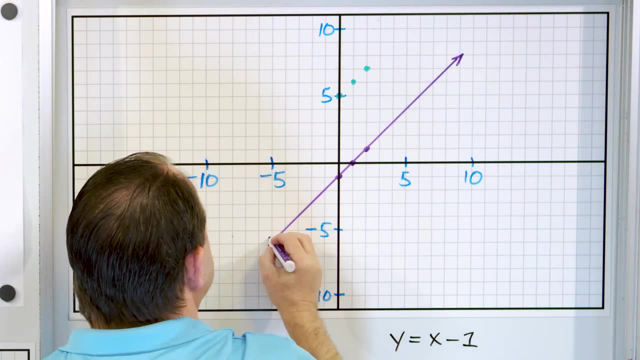 We're trying to get an idea of what's going on here as cleanly as we can, So we'll draw this guy, something like that, and that goes through all three of these points. So there is a line that goes on and on, forever, to infinity, in both directions. 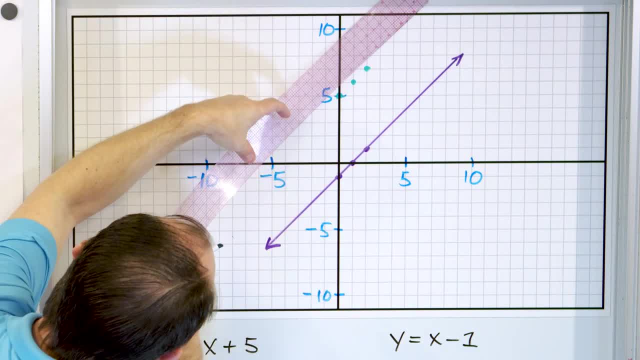 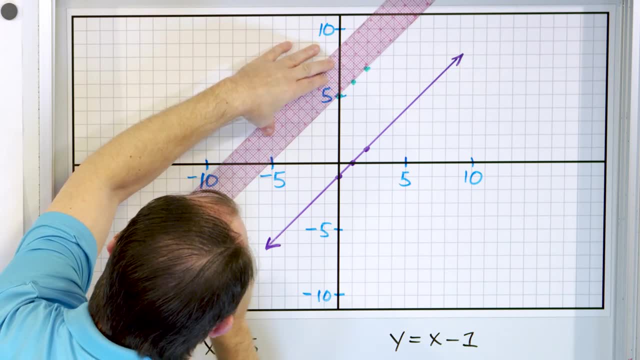 And then we're going to draw this one, which I think you can probably see what's going to happen. Let's see if I can get it lined up exactly. All right, something like that: Let's take a look at this, Draw this guy right here. 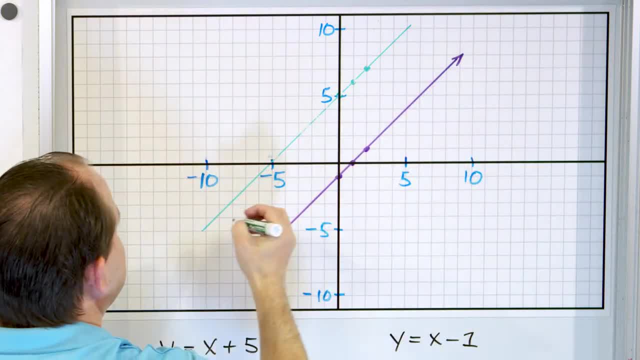 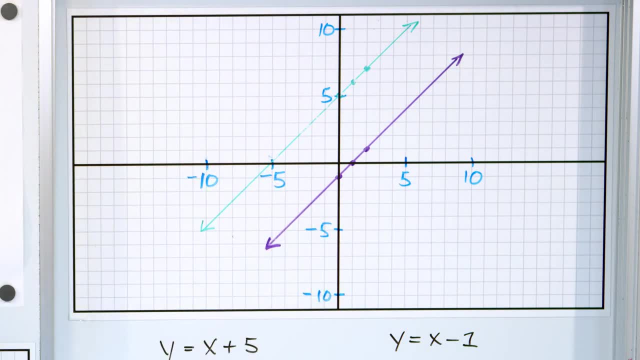 All right, Where is the intersection point of these two lines? I messed up my line when I pulled the thing off. You get the idea It goes like this: Where is the intersection point of these two lines? Well, there is no intersection point. 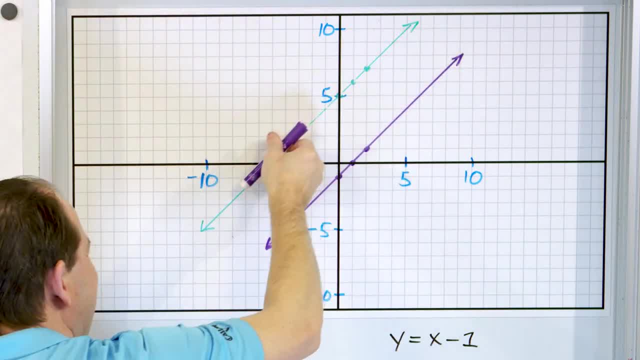 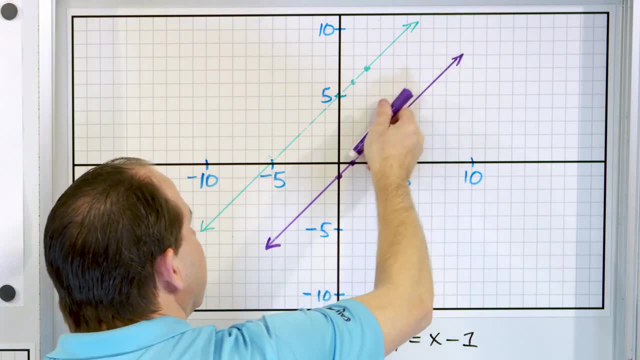 This line, this green one, is going to go on and on, forever, to infinity, to the end of the universe, along this direction. And this purple one is going to go on and on, forever, to the end of the universe, never stopping along this direction. 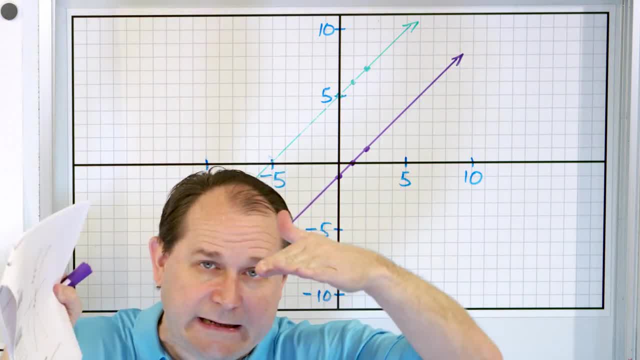 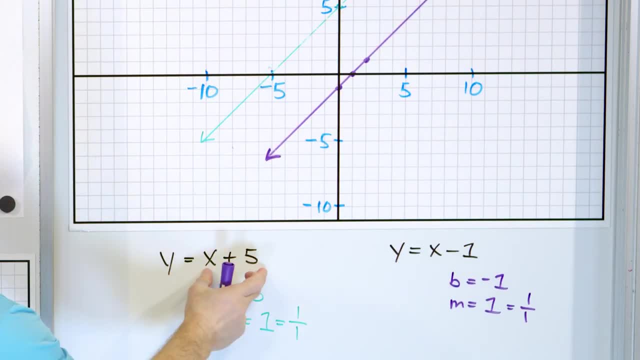 But these two lines will never, ever cross. Now, from our graph and this tiny little window we're looking at, it looks like they never cross, But mathematically you know that they're never going to cross. Why? Because this guy has a slope of one. 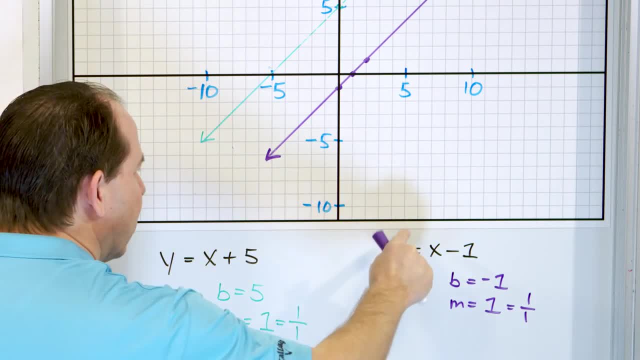 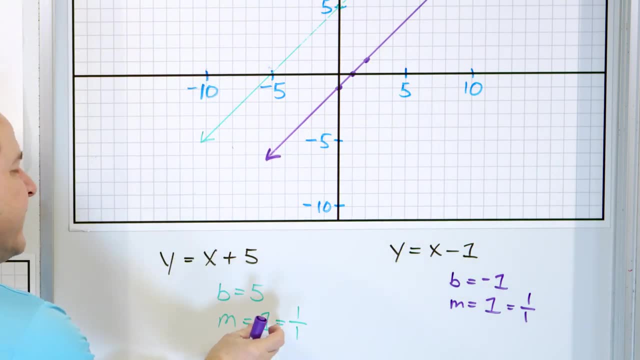 That means rise over, run Up and over is always up and over, up and over one over one. But the slope of this one is exactly the same thing: Up and over one, one, one, one. So because the slope of this is one and the slope of this is one, you know they have to. 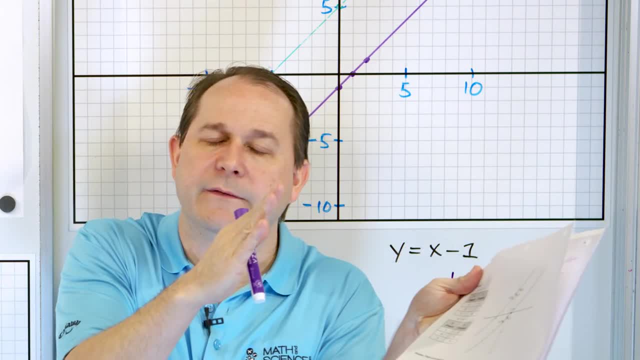 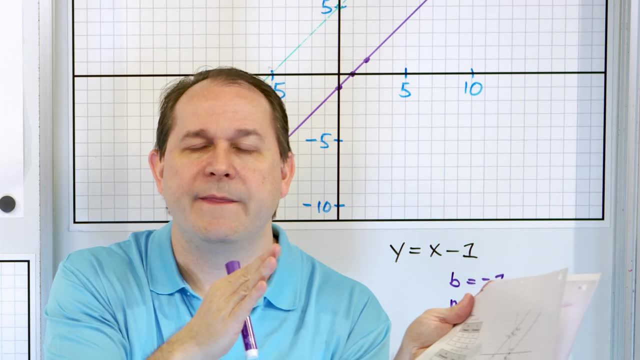 be parallel because the slope is telling you how tilted the line is. If both lines are tilted- and they're not on top of each other, but they're tilted the exact same angle, The same direction- then they can never cross, Because this line and this line are always going to be going rise over, run one over. 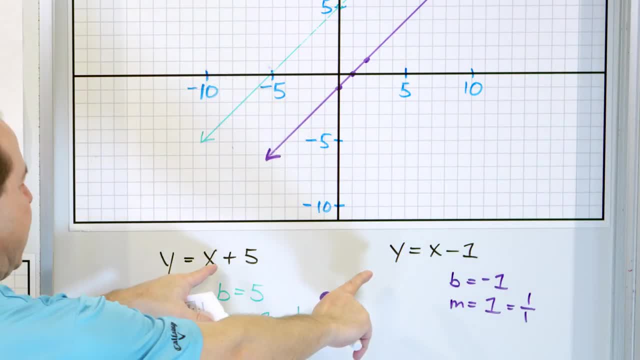 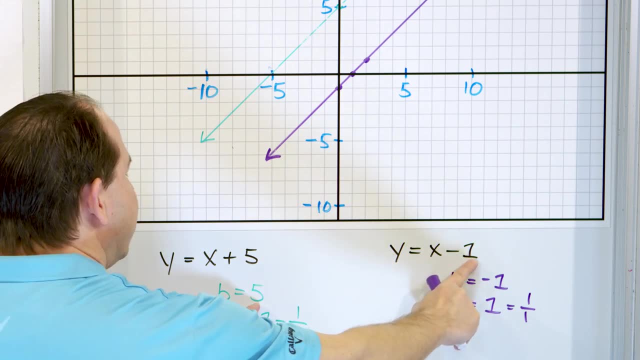 one same direction forever. The only actual difference between these is the y-intercept. So the slope is the same, but the y-intercept is different. The y-intercept is up at five and the y-intercept here is down at negative one. 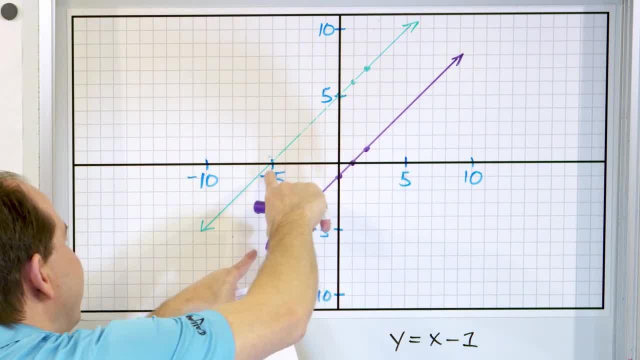 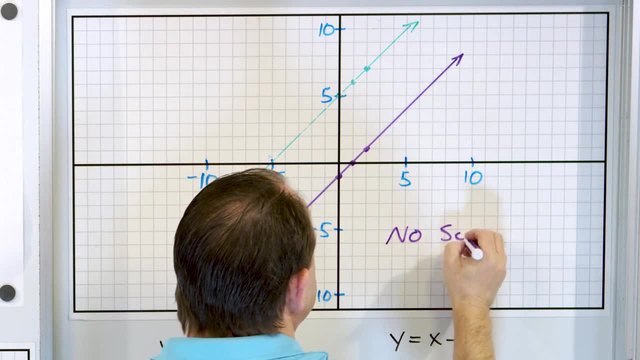 Y-intercept up at five, y-intercept at negative one. But from those starting points the slope means that since they're the same, they will never cross. So what you say Is that there is no solution And no solution happens when the two lines have the same slope. 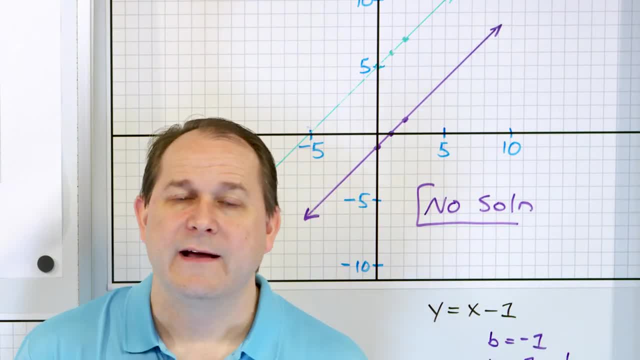 So even if you don't graph it, you know that they're going to be no solution if they have the same slope. So that's something to look for. But even if you forget, just graph them and you'll see that they're parallel. 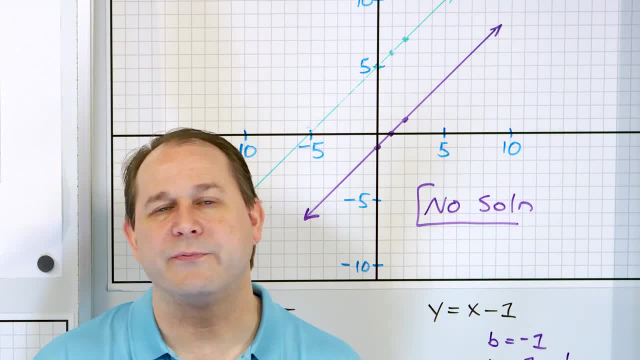 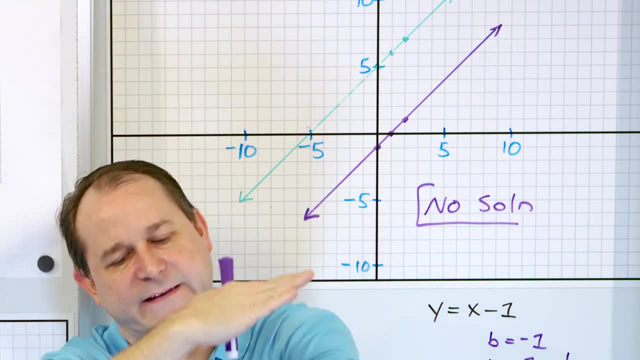 Another way of saying this is: you know that two lines are parallel. if the slopes are the same, It doesn't matter the y-intercept, that just tells you how up and down it crosses the y-axis. But if the slopes are the same,